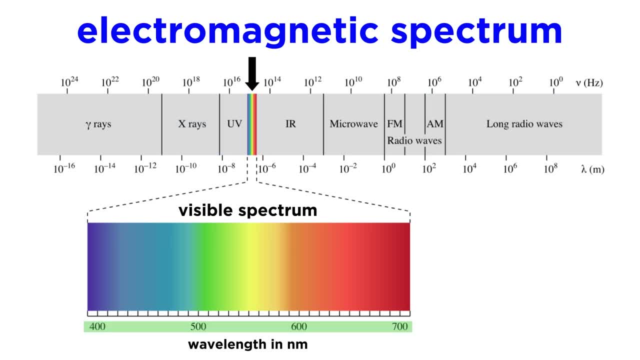 and radio waves and x-rays and all the rest. It just happens to have a wavelength between about 400 and 700 nanometers. This is the portion of the electromagnetic spectrum that we have been talking about for a long time. This is the portion of the electromagnetic spectrum that we have been talking about for. 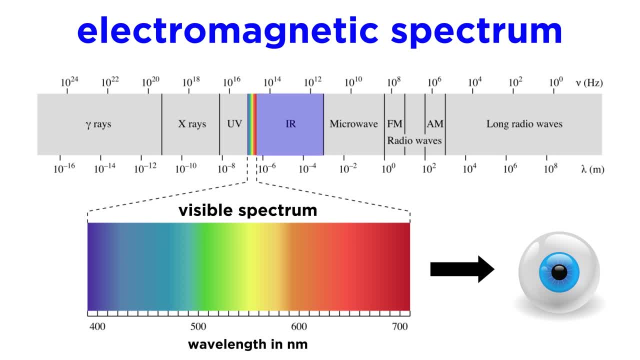 a long time and we have evolved the ability to perceive. If the wavelength is just a bit longer in the infrared portion, our eyes can't pick it up. A little shorter in the ultraviolet range, again we can't pick it up. 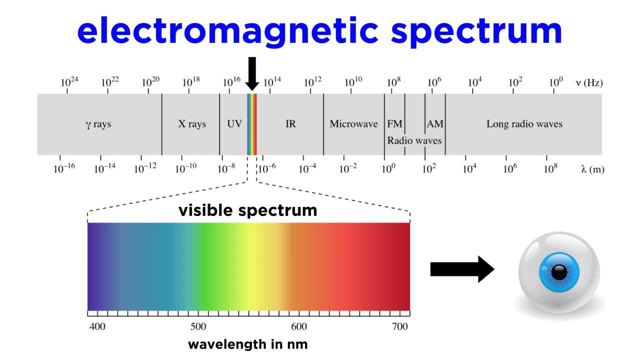 But right in this thin band, we are in business. Other species have slightly different ranges to work with, but this one is ours. Within that range, the specific wavelength determines the color of the light and the intensity determines the brightness of the light. 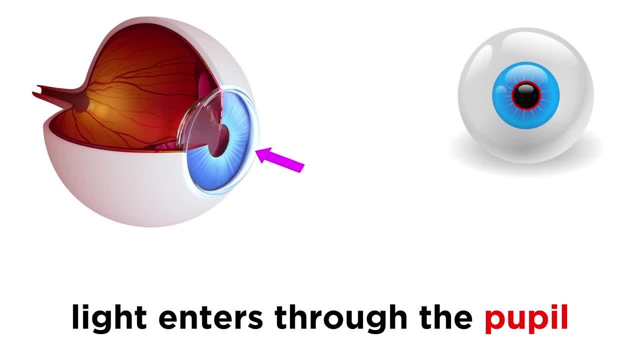 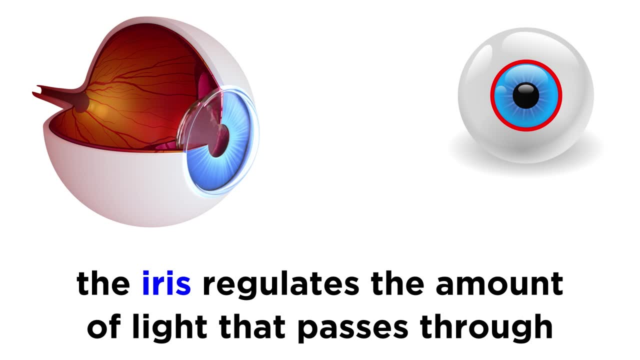 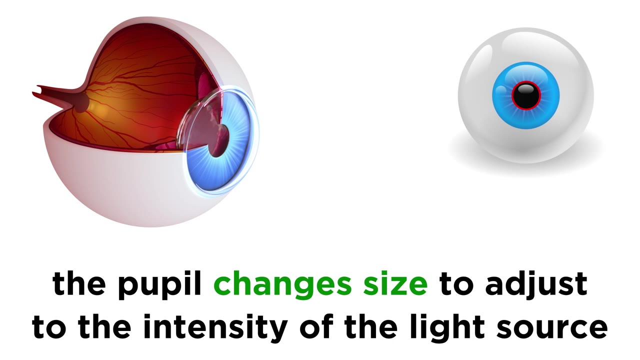 The intensity determines the brightness of the light. The intensity determines the brightness of the source. Light passes through the pupil to enter the eye. The iris or the colored part surrounding the pupil regulates the amount of light that passes through. This can be seen when the pupil changes size to adjust to the intensity of available light. 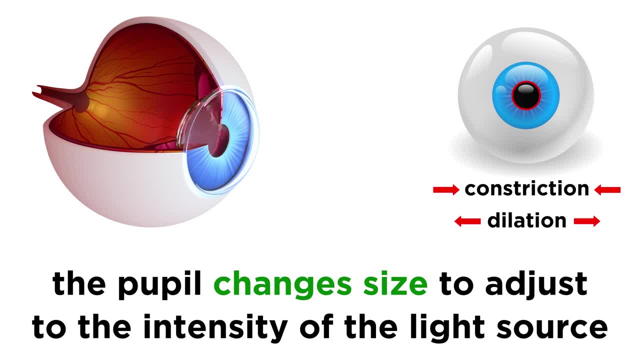 which we call constriction if it gets smaller and dilation if it gets bigger. Behind the pupil sits the lens which focuses the light onto the retina. The pupil then changes its size to adjust to the intensity of available light, which we call constriction if it gets smaller and dilation if it gets bigger. 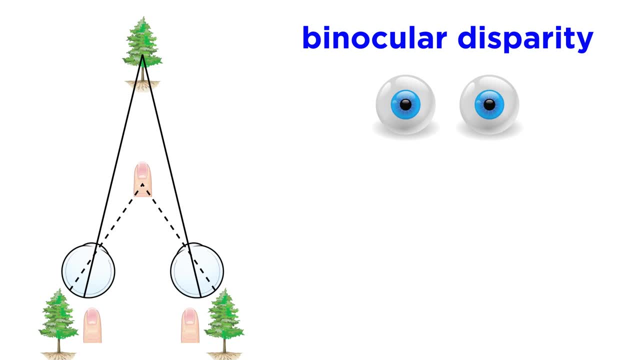 Behind the pupil sits the lens which focuses the light onto the retina. We do this with two eyes at once and the brain is able to interpret the binocular disparity, which is the difference in the position of a particular image on the two retinas. 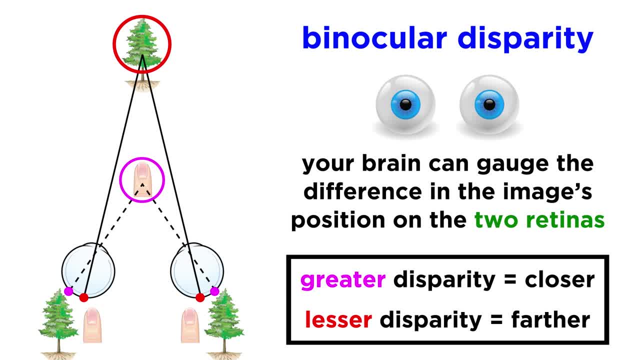 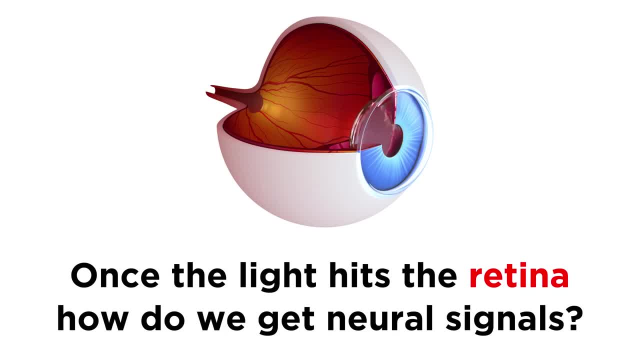 The greater the disparity, the closer the object is. so having two eyes is what gives us our depth perception. Now, the process by which light hitting the retina is converted into neural signals is quite complex, to say the least. To begin to understand this, let's zoom in a bit on the retina. 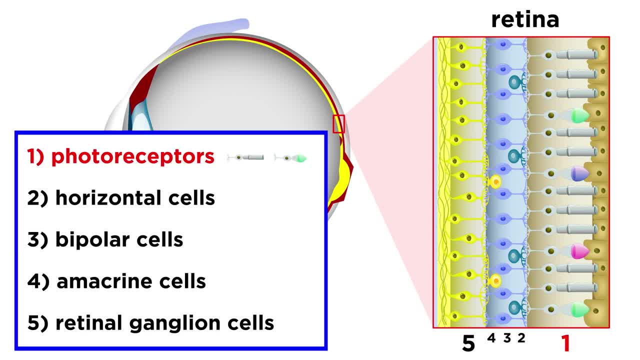 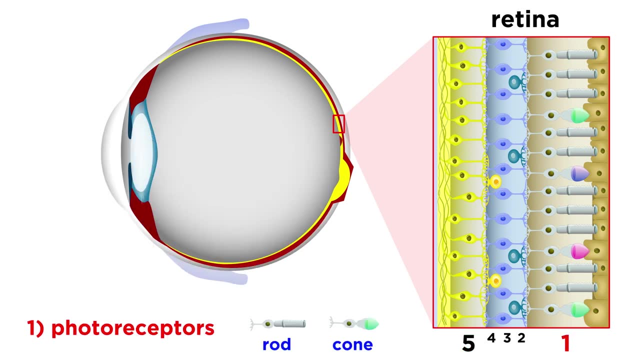 We see five layers of different types of neurons. There are receptor cells, horizontal cells, bipolar cells, amacrine cells and retinal ganglion cells. Interestingly enough, the photoreceptors, which are referred to as rods and cones, are 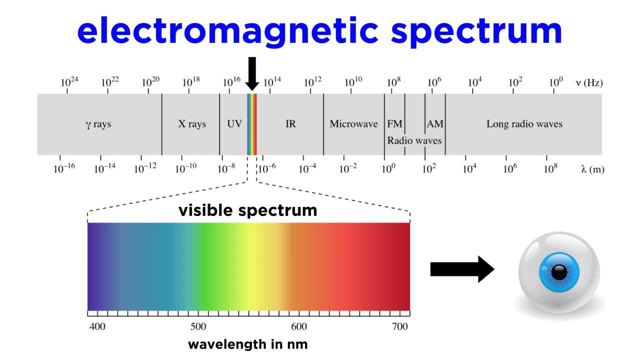 But right in this thin band, we are in business. Other species have slightly different ranges to work with, but this one is ours. Within that range, the specific wavelength determines the color of the light and the intensity determines the brightness of the light. 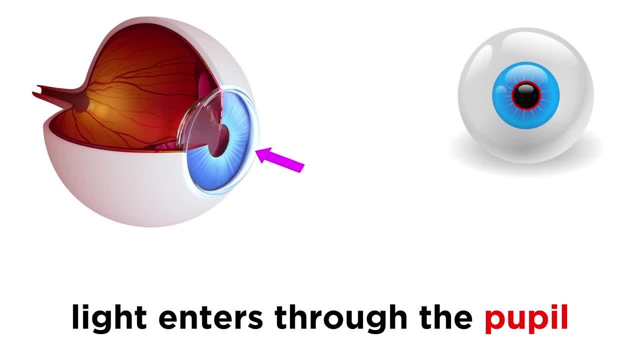 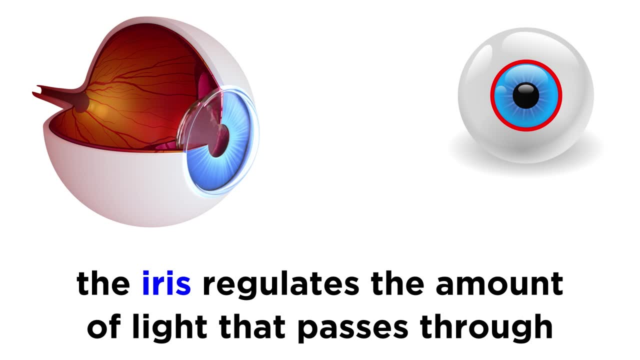 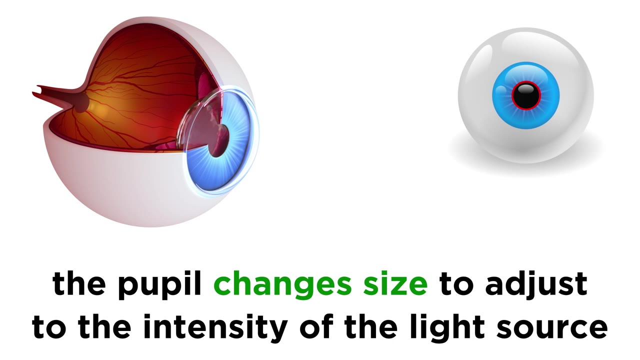 The intensity determines the brightness of the light. The intensity determines the brightness of the source. Light passes through the pupil to enter the eye. The iris or the colored part surrounding the pupil regulates the amount of light that passes through. This can be seen when the pupil changes size to adjust to the intensity of available light. 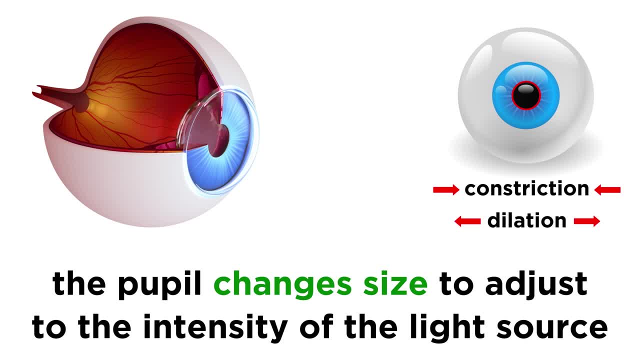 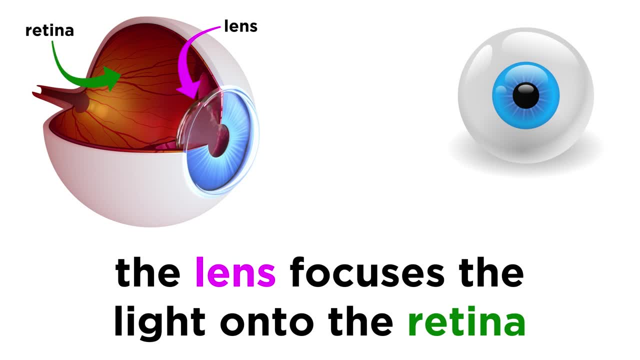 which we call constriction if it gets smaller, and dilation if it gets bigger. Behind the pupil sits the lens which focuses the light onto the retina. The lens is the lens that focuses the light onto the retina. The lens is the lens that focuses the light onto the retina. 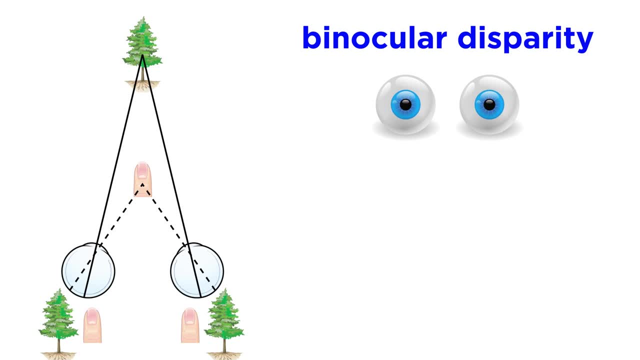 The lens is the lens that focuses the light onto the retina. We do this with two eyes at once, and the brain is able to interpret the binocular disparity, which is the difference in the position of a particular image on the two retinas. 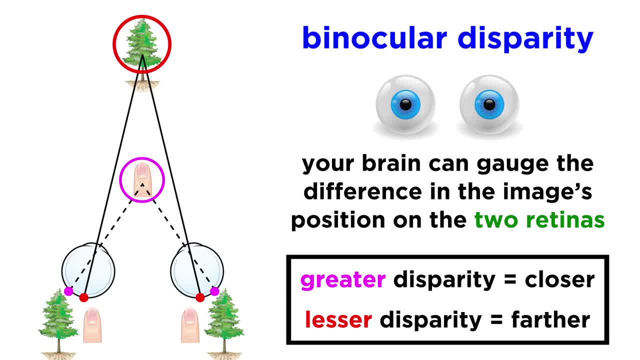 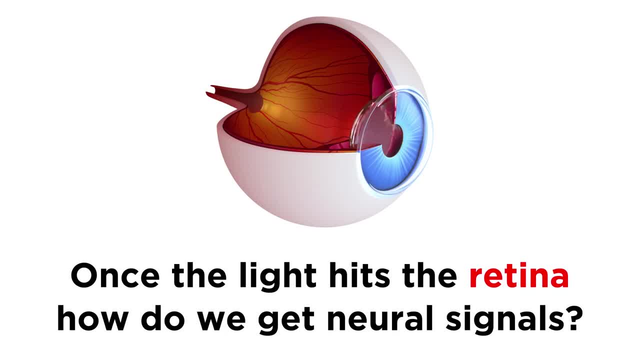 The greater the disparity, the closer the object is. so having two eyes is what gives us our depth perception. Now, the process by which light hitting the retina is converted into neural signals is quite complex. To begin to understand this, let's zoom in a bit on the retina. 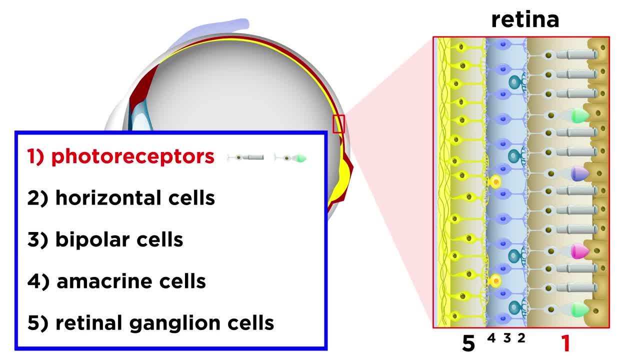 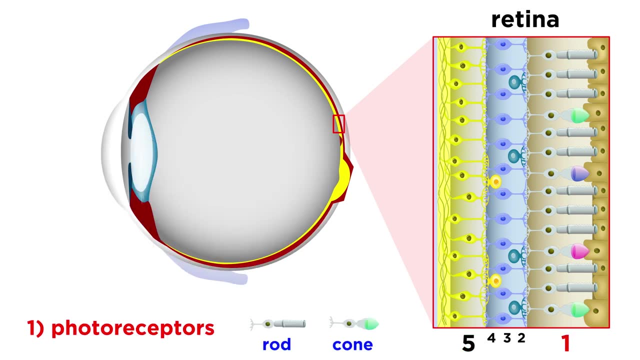 We see five layers of different types of neurons. There are receptor cells, horizontal cells, bipolar cells, amacrine cells and retinal ganglion cells. Interestingly enough, the photoreceptors, which are referred to as rods and cones, depending on their shape, are located at the back of the eyeball, so light must reach these first. 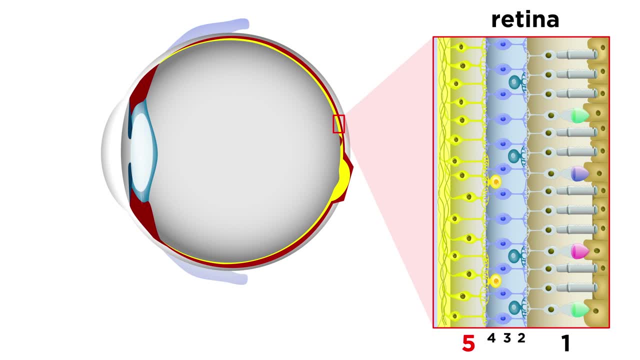 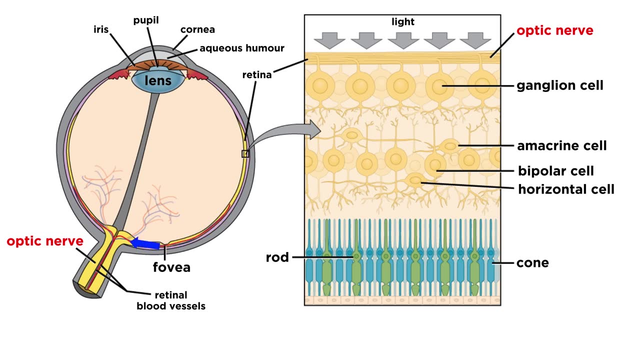 and then the resulting signals propagate out towards the retinal ganglion cells. The signal continues along the axons from these retinal ganglion cells to leave the eye, and the disruption in the receptor layer that this bundle of axons creates is what results. 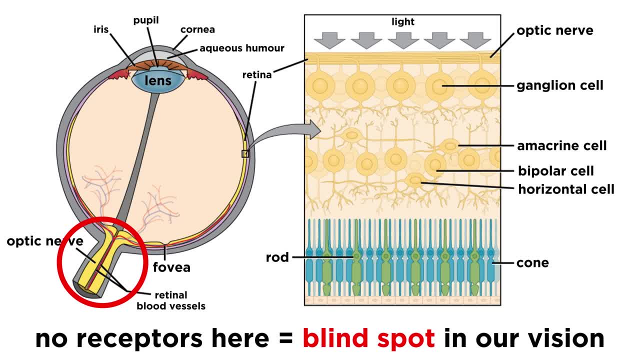 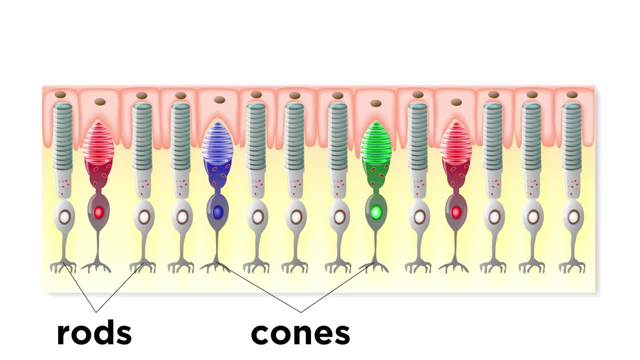 in a blind spot in our vision. Let's now get a closer look at these rods and cones. Let's start with the retina. Let's start with the retina. They are called cones. Looking at their shapes, the origin of their names becomes quite obvious. 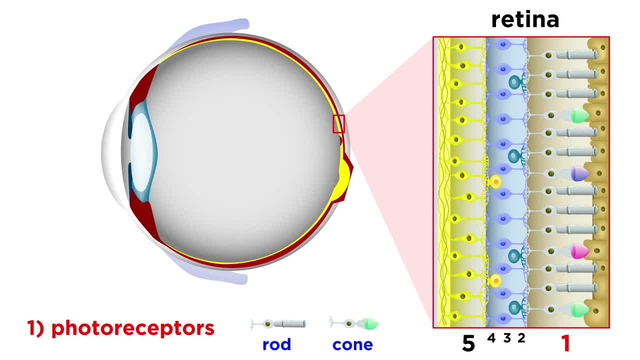 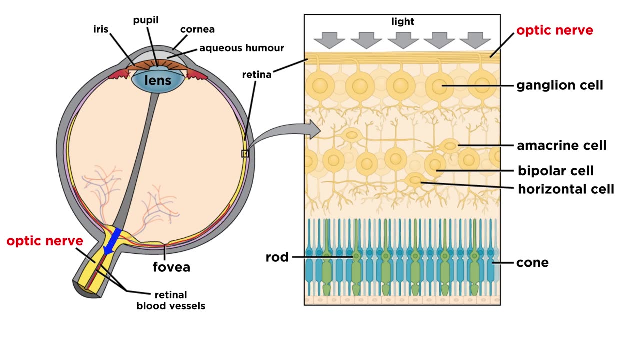 called photoreceptors. Photoreceptors, depending on their shape, are located at the back of the eyeball, so light must reach these first, and then the resulting signals propagate out towards the retinal ganglion cells. The signal continues along the axons from these retinal ganglion cells to leave the 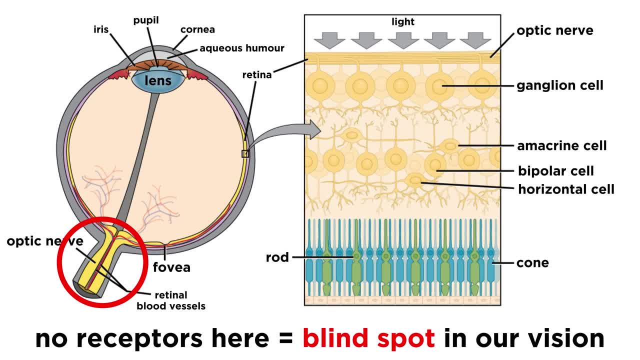 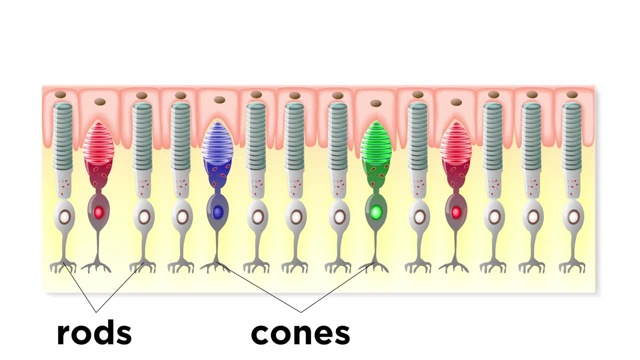 eye and the disruption in the receptor layer that this bundle of axons creates is what results in a blind spot in our vision. Let's now get a closer look at the retina. You can see that they are made of real metal and they are filled with the maximum amount. 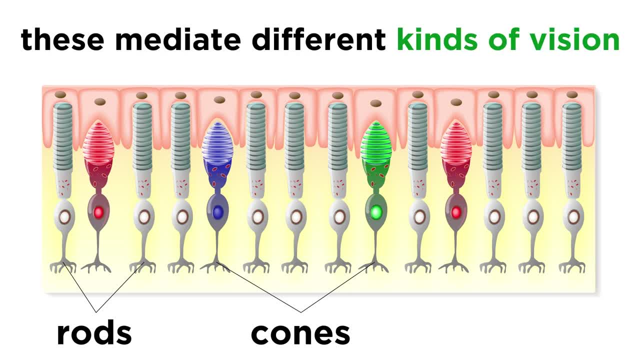 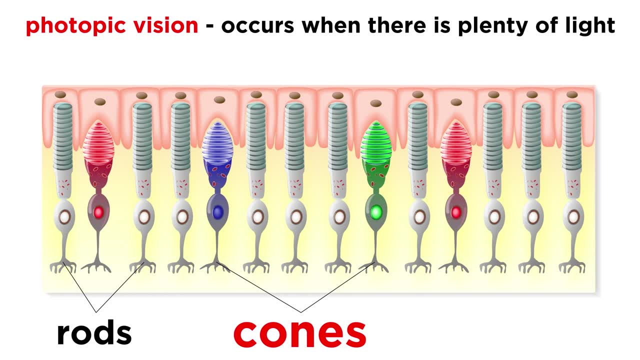 of light and the maximum amount of light produced by the retina. The main reason for those lights is the lack of light and therefore the position of the retina. The most common reason is that the light is too bright. As with plastic surgery, the light is more bright and the presence of light is less. 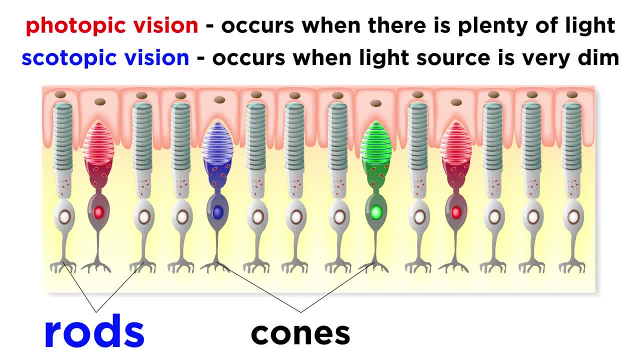 than the appearance. Now, the red lines on the retina are the light and the light is the light? not enough light to excite the cones. This is mediated by rods and it produces a kind of perception that lacks certain details. This is better understood when looking at how these neurons converge. 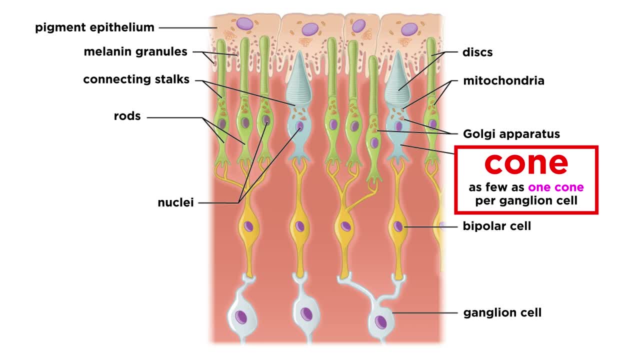 Looking at cones, only a few of these converge onto one retinal ganglion cell, so the input received here is from just a few photoreceptors. By contrast, several hundred rods converge onto a single retinal ganglion cell, so the input received in this case is from a great many photoreceptors. 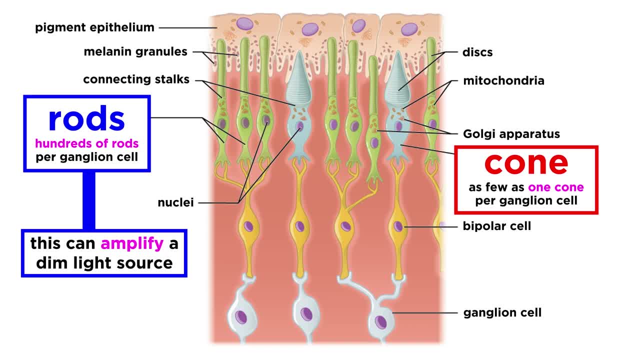 This is why the rods can take a very dim light source and amplify the stimulation, whereas this would not work with cones. This system trades sensitivity for acuity, because an amplified signal means the information will be received, but it can't be pinpointed. 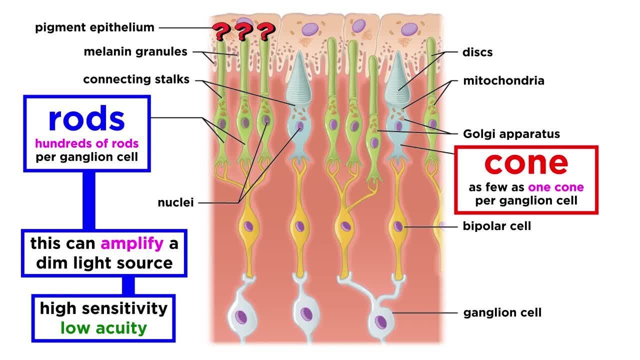 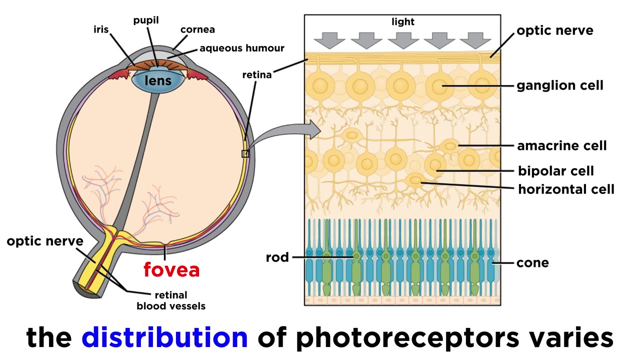 So it is less clear where the signal is coming from. With cones, there is less sensitivity, but there is little ambiguity. The stimulus is coming from a distinct place. so with a brighter light source, this is more effective In terms of the distribution of photoreceptors on the retina. we must be aware of the fovea. 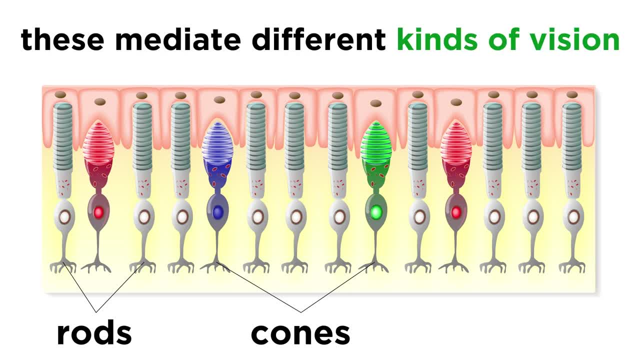 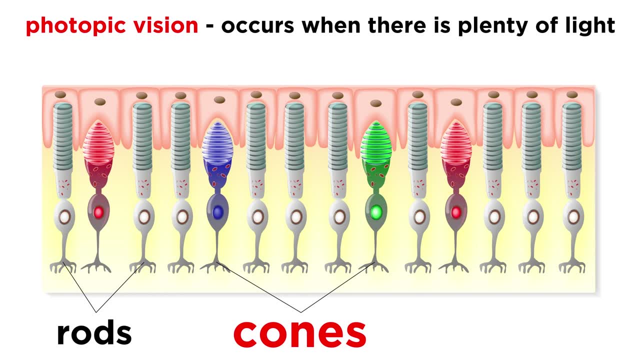 So how do they differ? As it happens, they mediate different kinds of vision. Photopic vision is what happens when there is plenty of light, which allows us to perceive our surroundings in great detail. This is mediated by cones. Scotopic vision is what happens when things are very dim and there is not enough light. 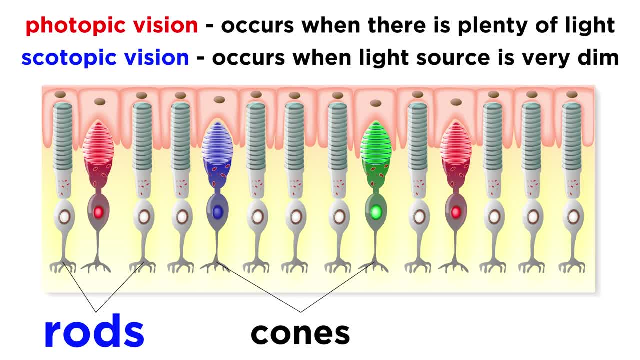 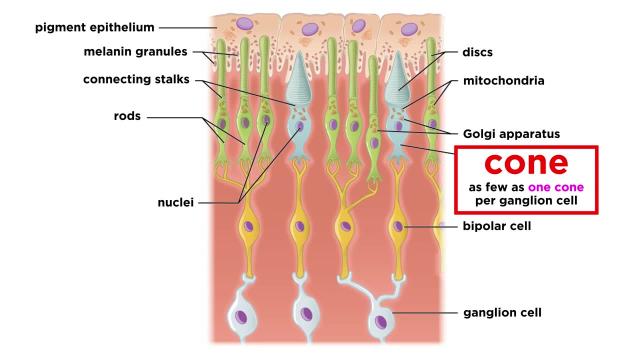 to excite the cones. This is mediated by rods and it produces a kind of perception that lacks certain details. This is better understood when looking at how these neurons converge, Looking at cones, only a few of these converge onto one retinal ganglion cell. so the input 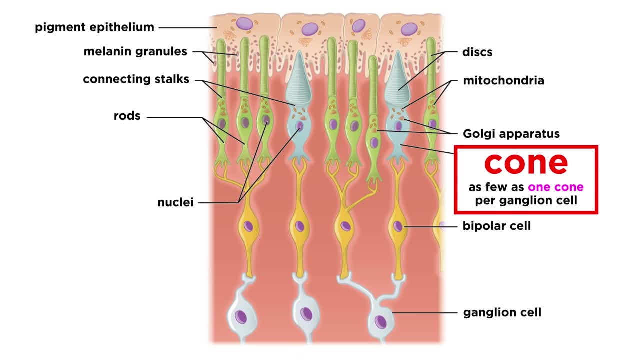 received here is from just a few photoreceptors. By contrast, several hundred rods converge onto a single retinal ganglion cell, so the input received in this case is from a great many photoreceptors. This is why the rods can take a very dim light source and amplify the stimulation, whereas 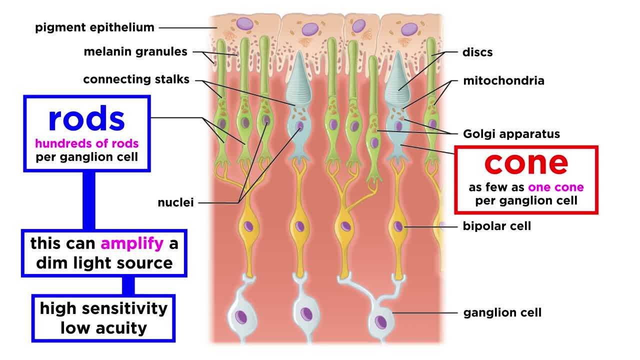 this would not work with cones. This system trades sensitivity for acuity, because an amplified signal means the information will be received, but it can't be pinpointed. With cones, there is less sensitivity, but there is little ambiguity. The stimulus is coming from a distinct place. so with a brighter light source, this is more. 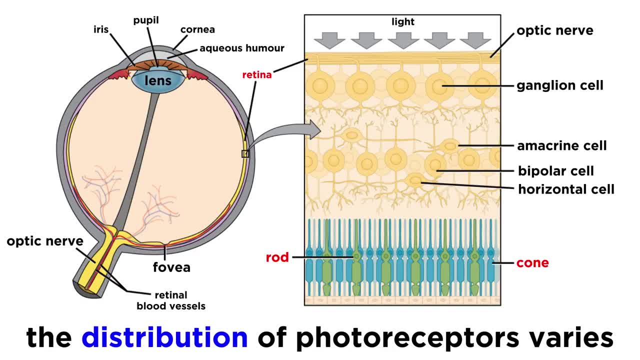 effective In terms of the distribution of photoreceptors on the retina. we must be aware of the fovea. The fovea, which means pit in Latin, is a small indentation at the center of the retina. in the retina, 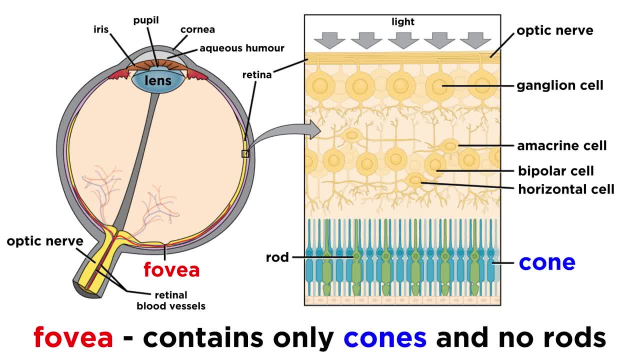 center of the retina and there are no rods at all in the fovea, only cones, Because this region is all cones. this is the part of the retina that specializes in high acuity vision, which means it can resolve small details. 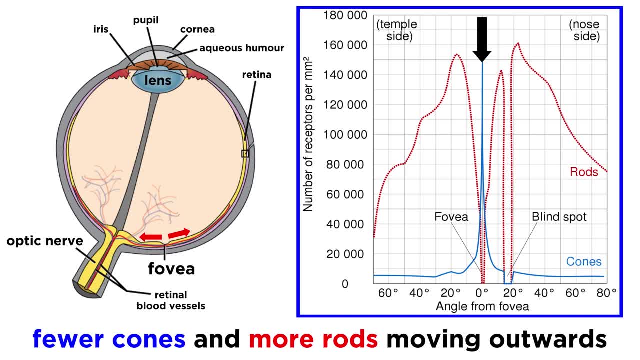 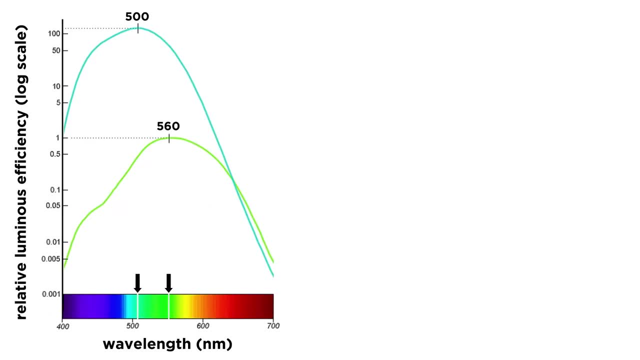 Then moving out from the fovea, there are fewer cones and many more rods. The rods reach a maximum at 20 degrees away from the fovea on either side and then begin to decline as well. The sensitivity towards particular wavelengths of light is slightly different for these two. 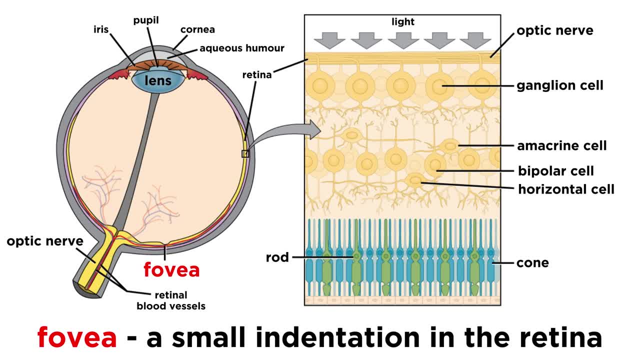 The fovea, which means pit in Latin, is a small indentation at the retina, At the center of the retina, And there are no rods at all in the fovea, only cones, Because this region is all cones. this is the part of the retina that specializes in. 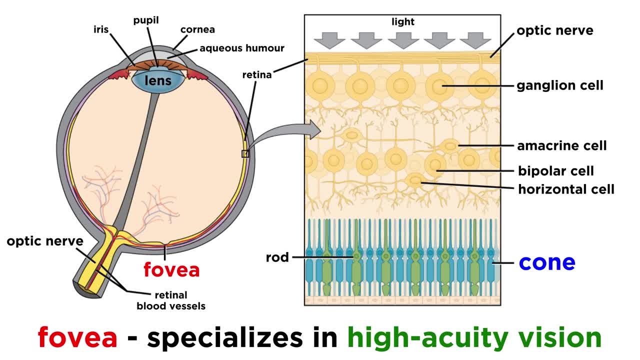 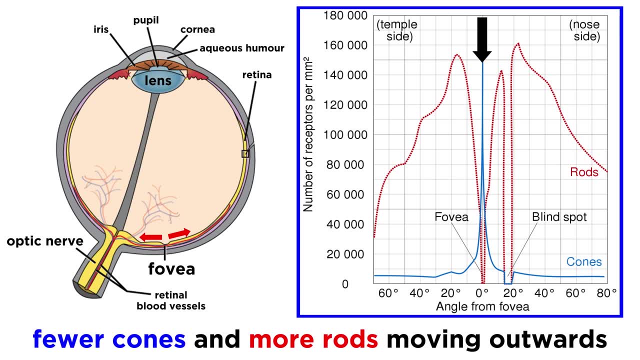 high acuity vision, which means it can resolve small details. Then, moving out from the fovea, there are fewer cones and many more rods. The rods reach a maximum at 20 degrees away from the fovea on either side and then begin. 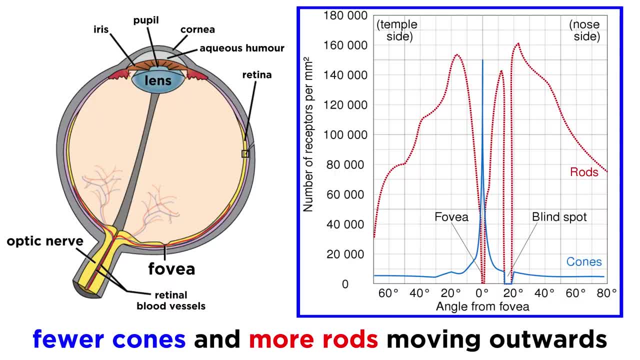 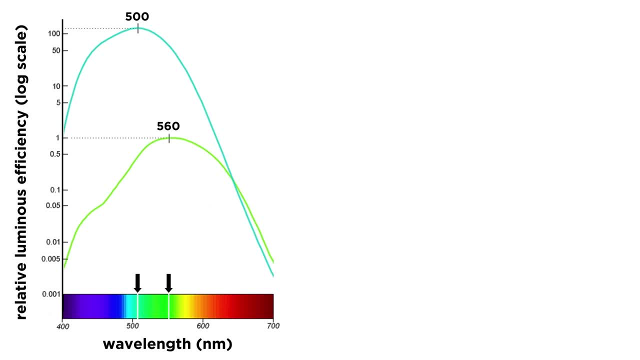 to decline as well. The sensitivity towards particular wavelengths of light is slightly different for these two receptor cells as well. With photopic vision and the cones, maximum sensitivity happens at around 560 nanometers, which is roughly yellow light. As it deviates from this, it will have to be more and more intense in order to be perceived. 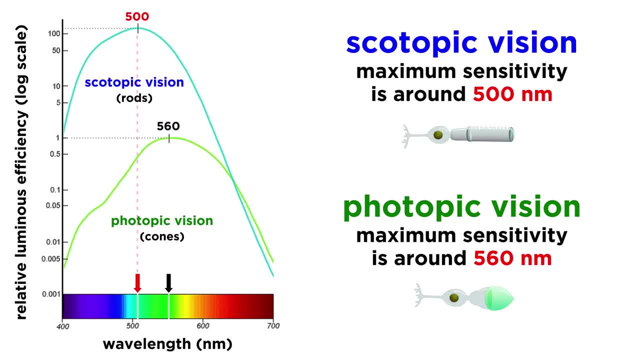 with the same brightness. With scotopic vision and the rods there is less sensitivity. The sensitivity towards particular wavelengths of light is slightly different for these two receptor cells as well. With photopic vision and the cones, maximum sensitivity happens around 500 nanometers. 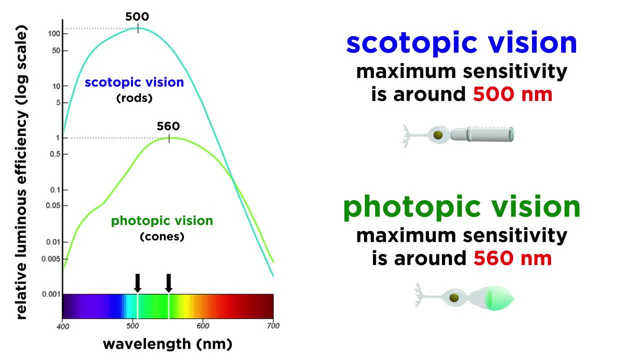 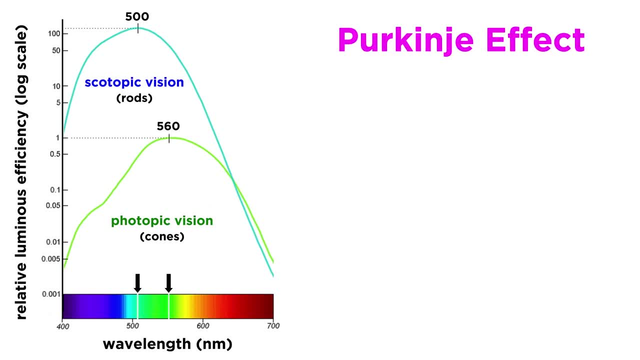 sort of a bluish-green light. As light dims and our eyes switch from photopic to scotopic vision, an interesting phenomenon can be observed that relates to this discrepancy in sensitivity, which is called the Purkinje effect. Yellow and red objects will appear brighter than green and blue ones, and as the light 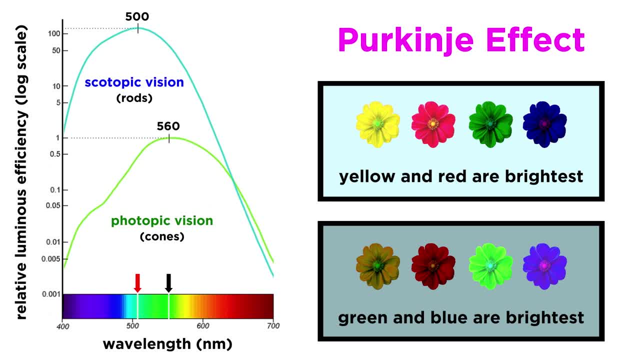 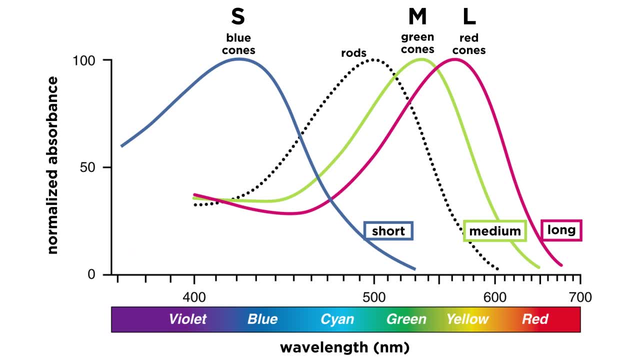 dims, this relative brightness will appear to reverse. To get even more specific with cones, we must understand that there are three cone types. These are red, green and blue, which are also called L, M and S, which stand for long. 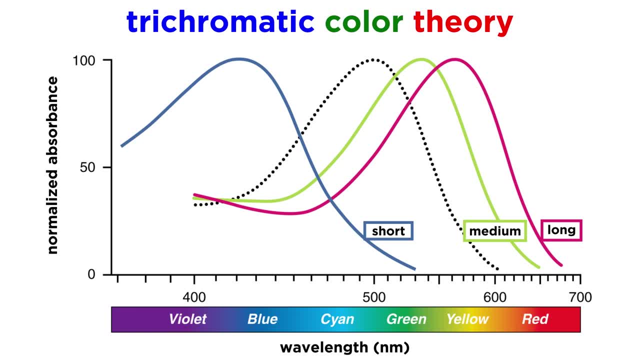 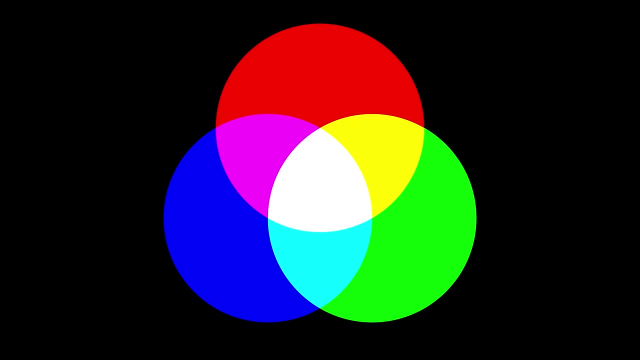 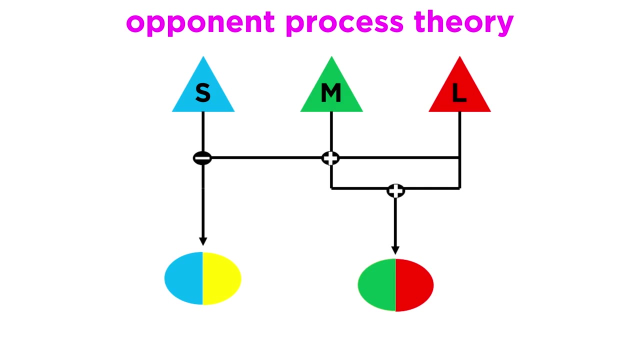 medium and short wavelength. Automatic color theory explains how differential activation of these three types is responsible for our perception of all colors. This is why a computer monitor can use only red, green and blue pixels to represent any color. This can be combined with opponent process theory, which outlines opponent systems that 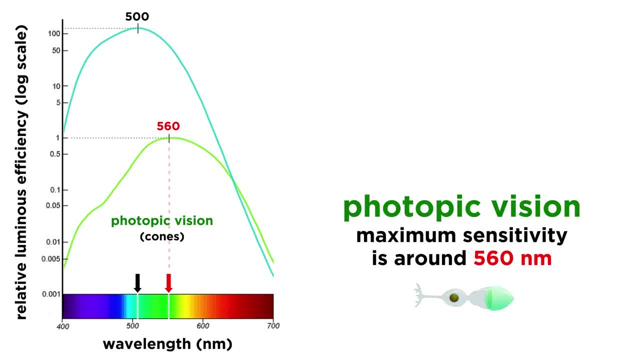 receptor cells as well. With photopic vision and the cones, maximum sensitivity happens at around 560 nanometers, which is roughly yellow light. As it deviates from this, it will have to be more and more intense in order to be perceived with the same brightness. 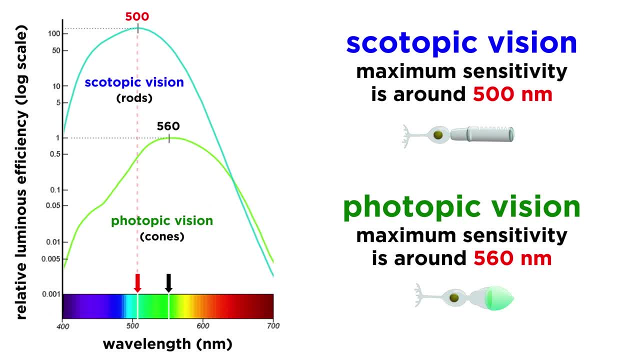 With scotopic vision it will have to be more intense in order to be perceived with the same brightness. With photopic vision and the rods, maximum sensitivity happens around 500 nanometers, sort of a bluish-green light As light dims and our eyes switch from photopic to scotopic vision- an interesting phenomenon. 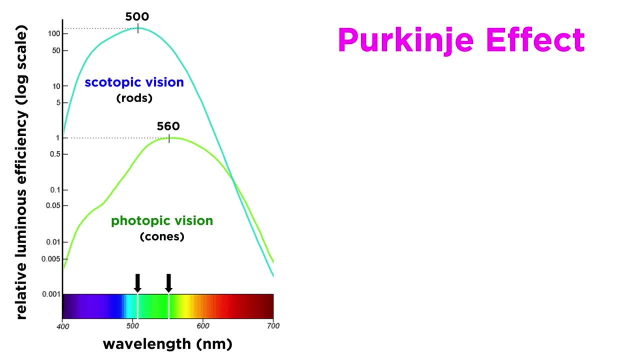 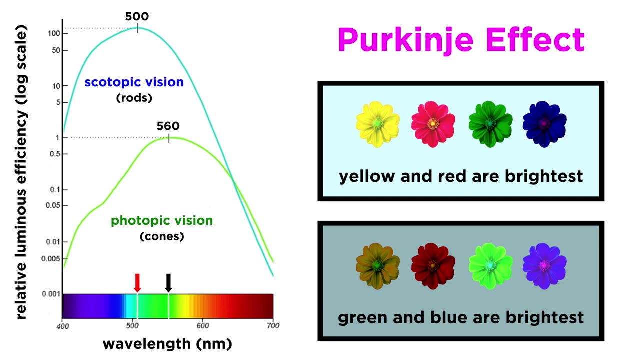 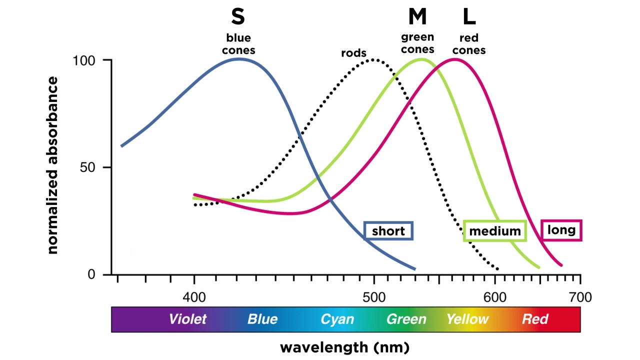 can be observed that relates to this discrepancy in sensitivity, which is called the Purkinje effect. Yellow and red objects will appear brighter than green and blue ones, and as the light dims, this relative brightness will decrease. To get even more specific with cones, we must understand that there are three cone types. 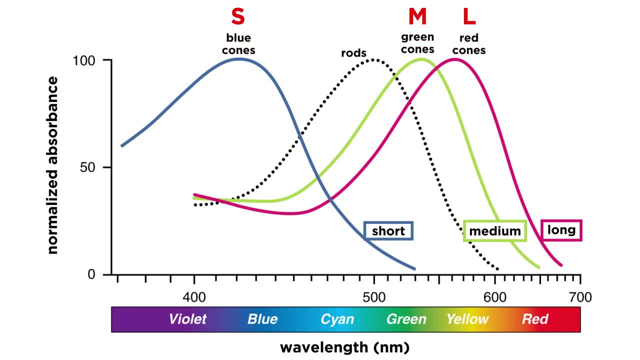 These are red, green and blue, which are also called L, M and S, which stand for long, medium and short wavelength. Trichromatic color theory explains how differential activation of these three types is responsible for our perception of all colors. 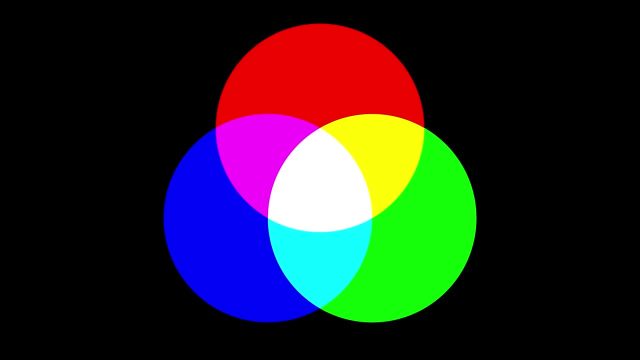 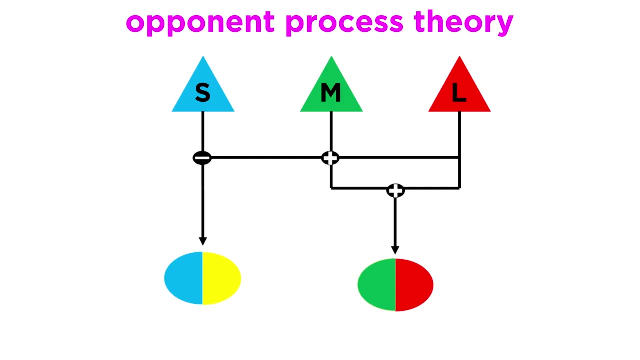 This is why a computer monitor can use only red, green and blue pixels to represent any color. This can be combined with opponent process theory, which outlines opponent systems that describe how the cones connect to the ganglion cells. In this model, a combination of excitatory and inhibitory responses controls what color. 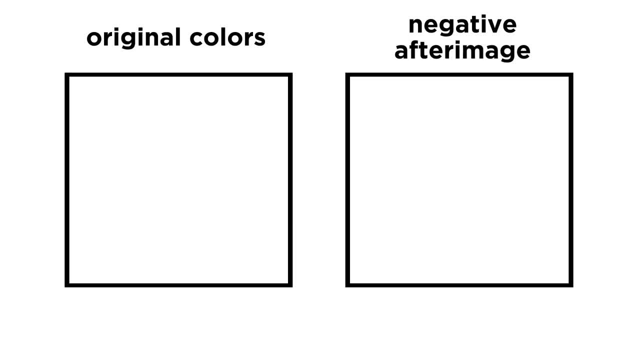 combinations can be seen. A ramification of this mechanism is the notion that the color combination of the cones is a motion of the negative afterimage that can be seen after staring at something for an extended period of time, whereby the afterimage is always the complementary color. 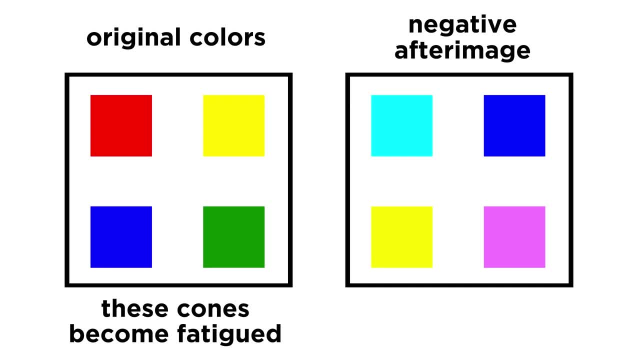 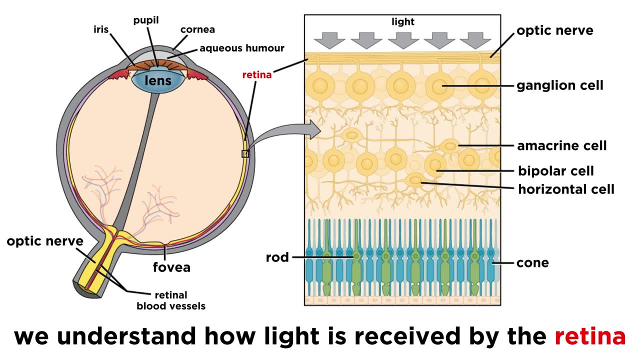 This is because staring at something of a particular color will cause certain cones to become fatigued, while others do not fire at all. so when shifting focus to a blank surface, only the opposing cells will fire. So now we have a basic grasp of how light is reflected. 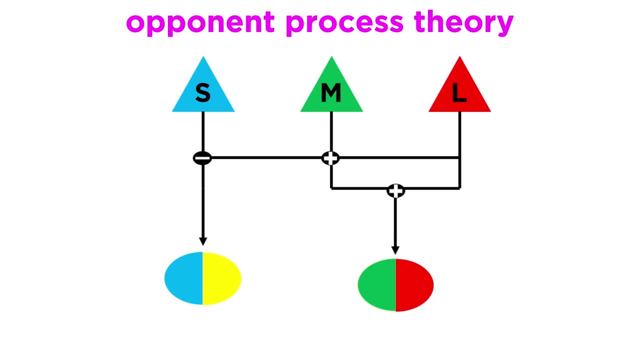 describe how the cones connect to the ganglion cells. In this model, a combination of excitatory and non-excitatory systems can be used to determine the color of the cones. The color combination of excitatory and inhibitory responses controls what color combinations. 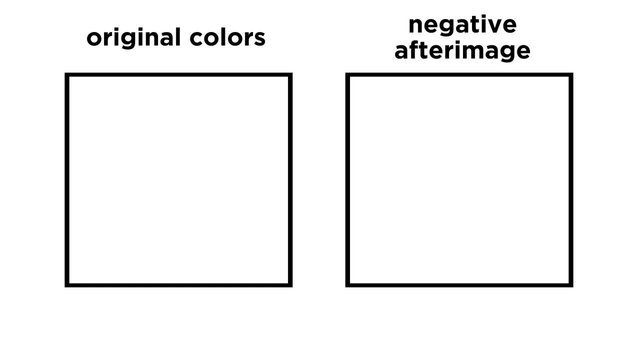 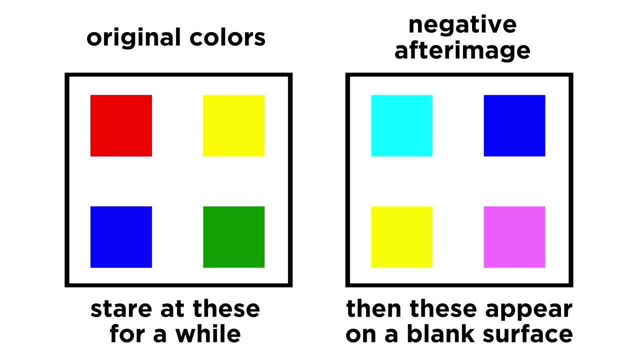 can be seen. A ramification of this mechanism is the notion of the negative afterimage that can be seen after staring at something for an extended period of time, whereby the afterimage is always the complementary color. This is because staring at something of a particular color will cause certain cones. 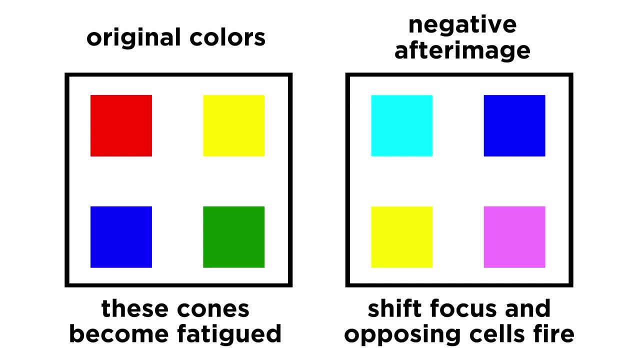 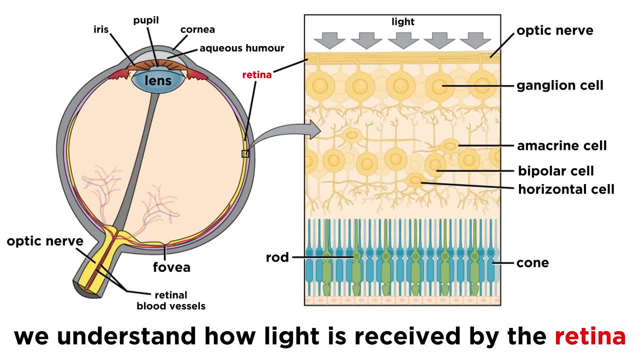 to become fatigued, while others do not fire at all. to a blank surface, only the opposing cells will fire. So now we have a basic grasp of how light is received by the retina, but how is this converted into information for the brain? Let's talk a bit about visual. 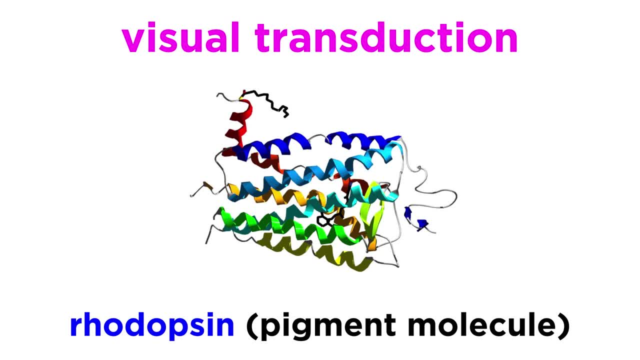 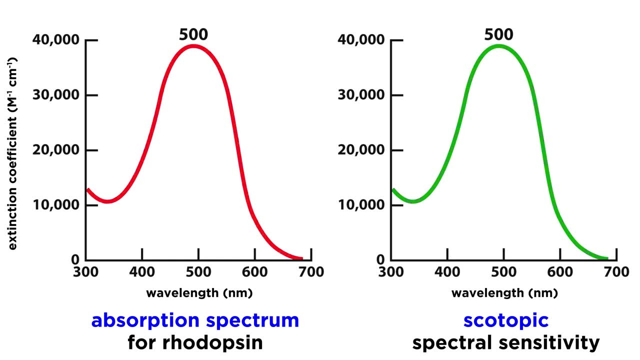 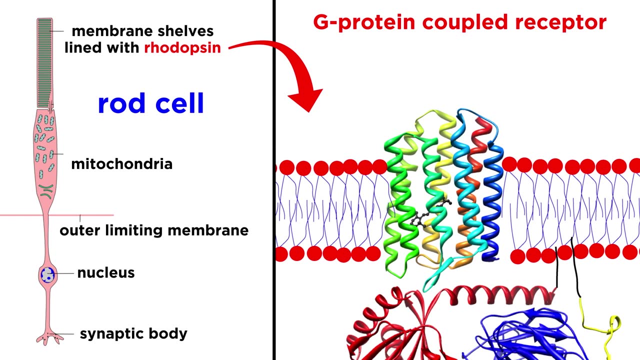 transduction. Take a look at this protein, a pigment molecule called rhodopsin. The absorption spectrum of this molecule is nearly identical to what we saw for the scotopic spectral sensitivity curve. This is no coincidence. This protein is a G-protein coupled receptor that is found in all of the rods, and the degree to 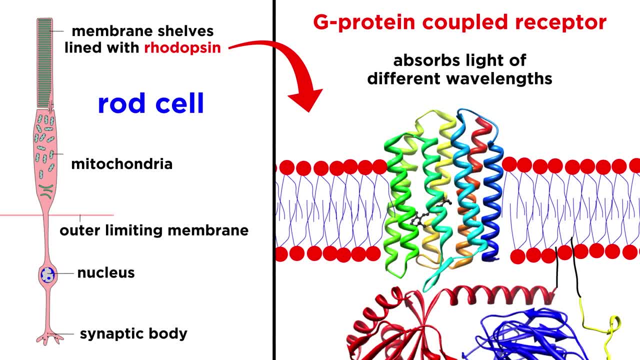 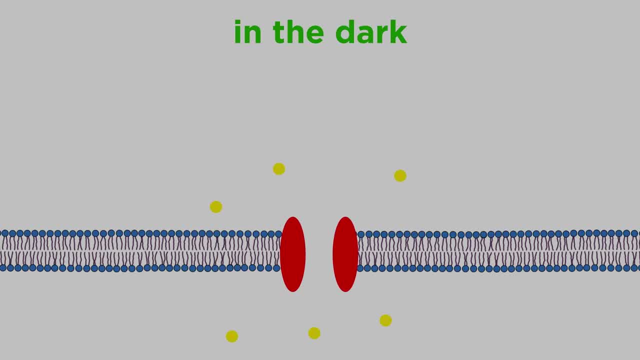 which it absorbs light of different wavelengths informs our ability to detect light of these wavelengths. The way this works is that in the dark, when rhodopsin is not activated by light, sodium channels are open, which keeps the rod slightly depolarized. 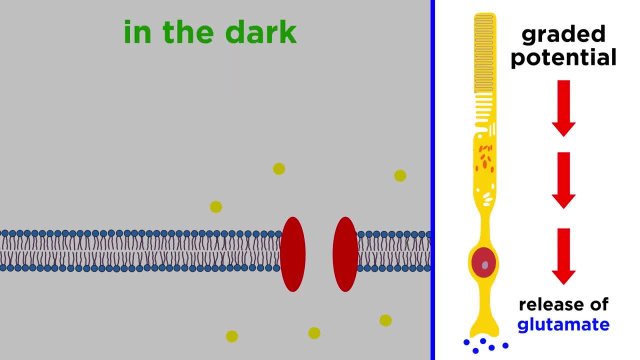 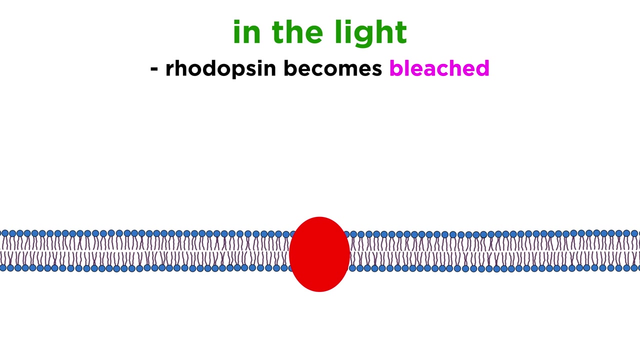 generating a graded potential, which results in the continuous release of glutamate. This is a neurotransmitter that has an inhibitory effect, keeping the bipolar cell hyperpolarized and inhibiting neurotransmitter release towards the ganglion cell. When exposed to light, rhodopsin becomes bleached, initiating a cascade of effects. 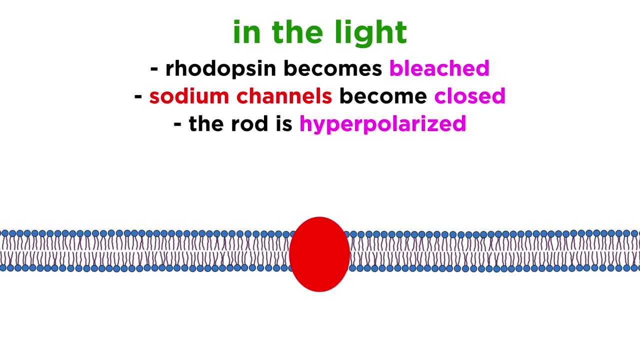 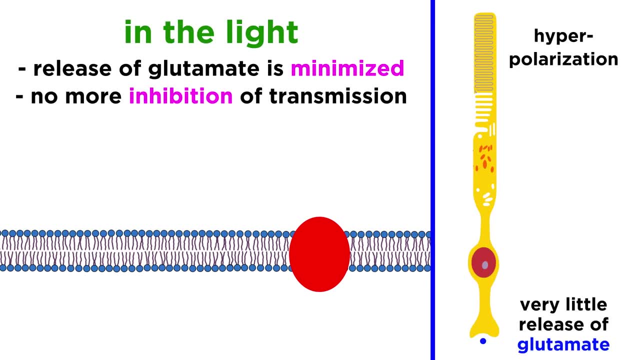 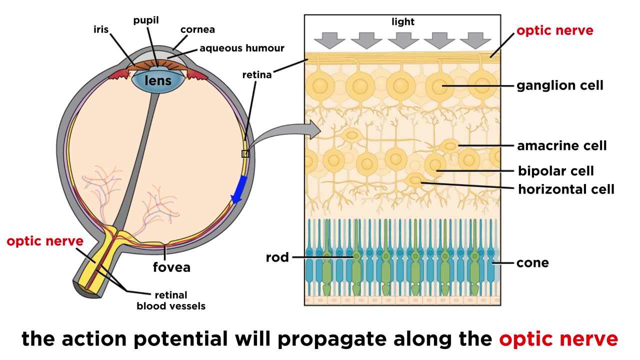 that results in the closure of the sodium channel. The rod becomes hyperpolarized and the release of glutamate is minimized, so the inhibition of signal transmission ceases. The bipolar cell can now depolarize and release neurotransmitters towards the ganglion cell, which will generate an action potential that can propagate. 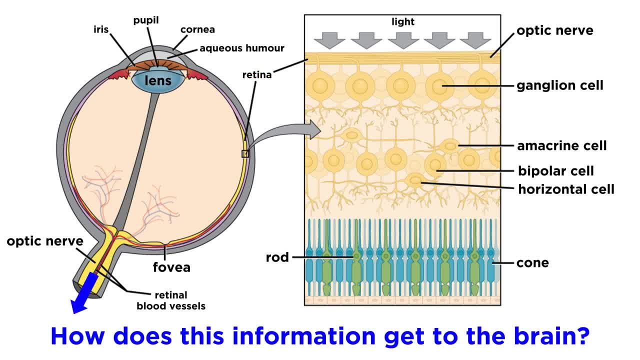 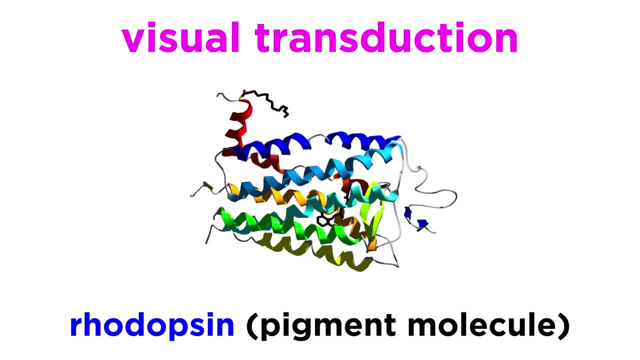 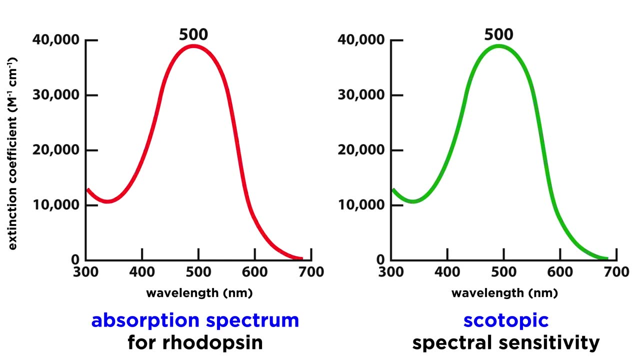 Let's take a look at some examples. Let's talk a bit about visual transduction. Take a look at this protein, a pigment molecule called rhodopsin. The absorption spectrum of this molecule is nearly identical to what we saw for the scotopic. 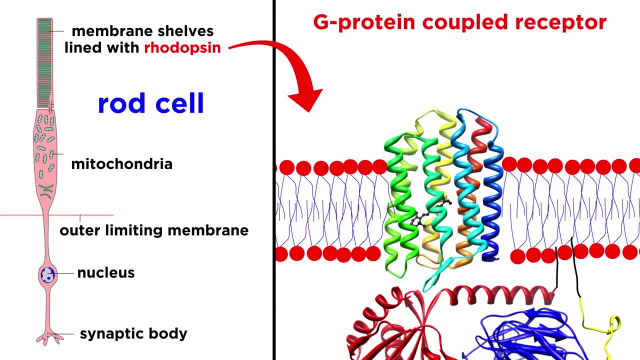 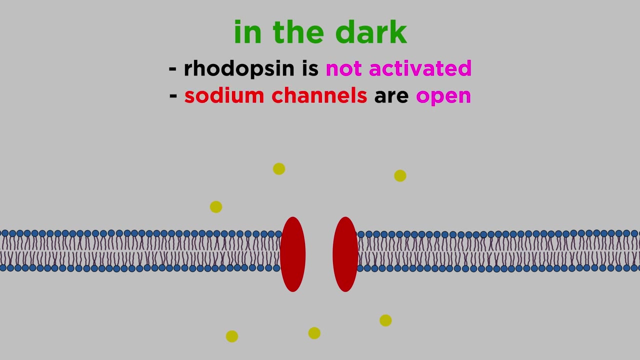 spectral sensitivity curve. This is no coincidence. this protein is a G-protein coupled receptor that is found in all of the rods, and the degree to which it absorbs light of different wavelengths informs our ability to detect light of these wavelengths. The way this works is that in the dark, when rhodopsin is not activated by light sodium. 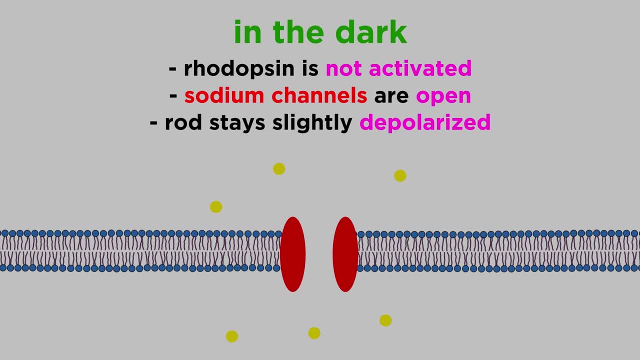 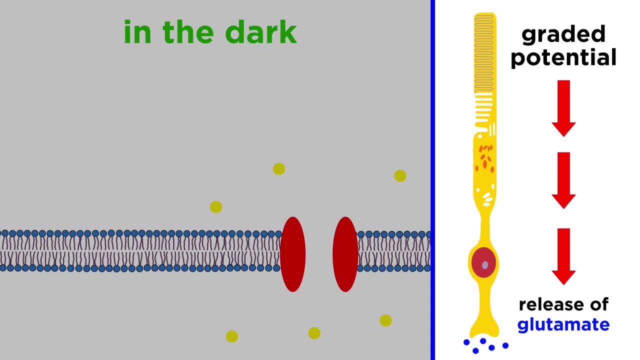 channels are open, which keeps the rod slightly depolarized, generating a graded potential which results in the continuous release of glutamate. This is a neurotransmitter that has an inhibitory effect, keeping the bipolar cell hyperpolarized and inhibiting neurotransmitter release towards the ganglion cell. 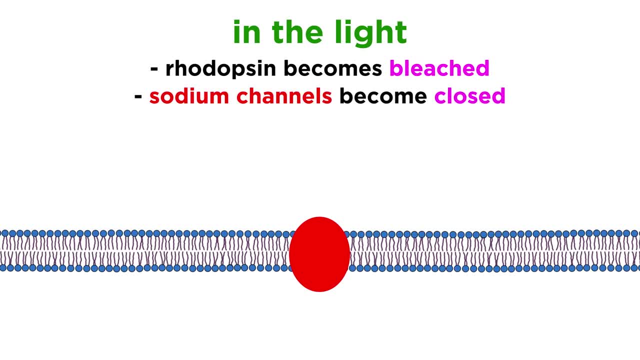 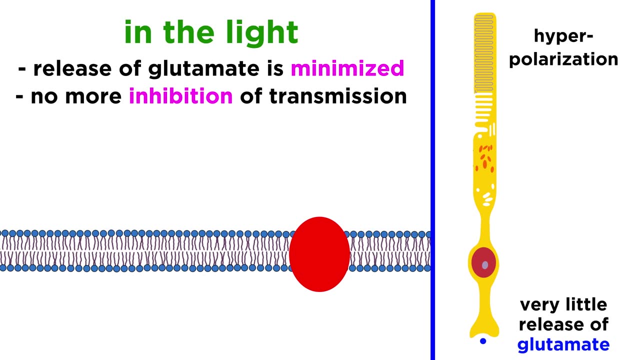 When exposed to light, rhodopsin becomes bleached, initiating a cascade of effects that results in the closure of the sodium channels. The rod becomes hyperpolarized and the release of glutamate is minimized, so the inhibition of signal transmission ceases. 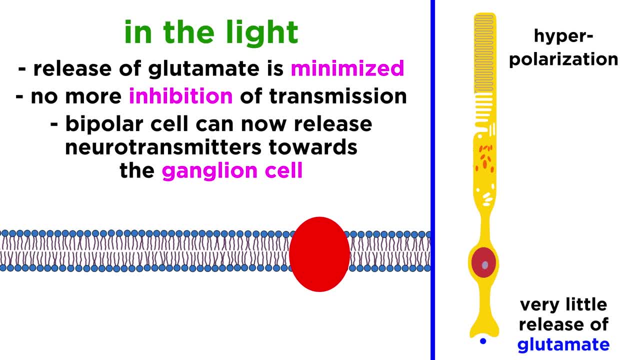 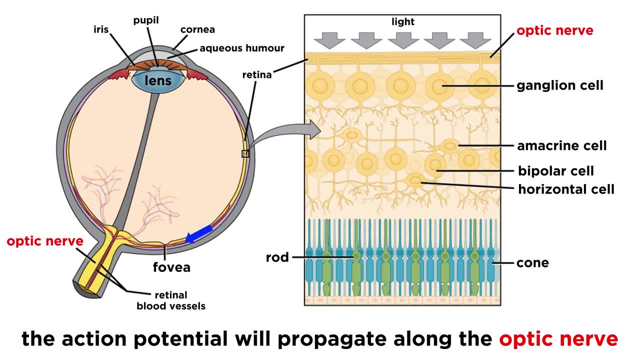 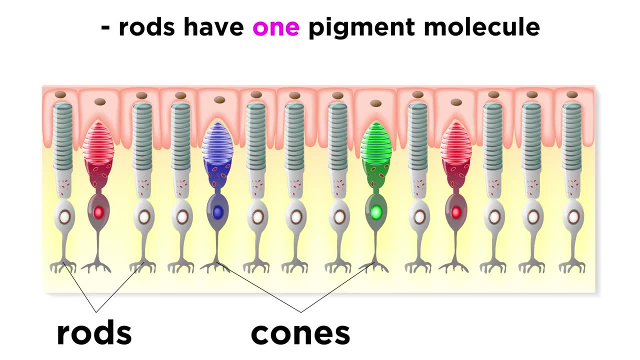 The bipolar cell can now depolarize and release neurotransmitters towards the ganglion cell, which will generate an action potential that can propagate along the optic nerve. We should note that rods contain just this one pigment, rhodopsin, while cones contain 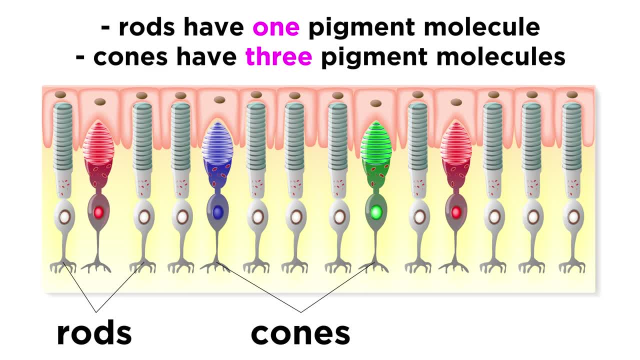 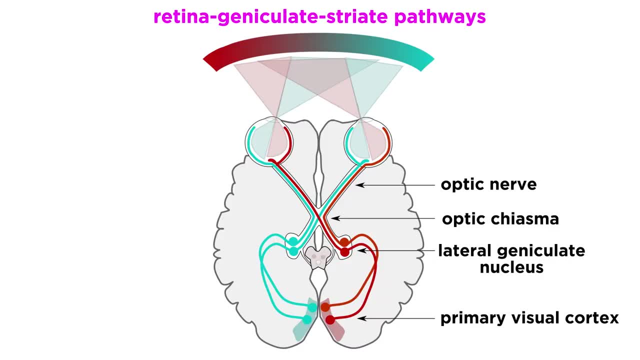 three which can act together in varying ways to allow for the perception of the signal of any color in the visible spectrum. Zooming out a bit: action potentials that start at the retinal ganglion cells will travel from the retina along retina-geniculate-striate pathways. 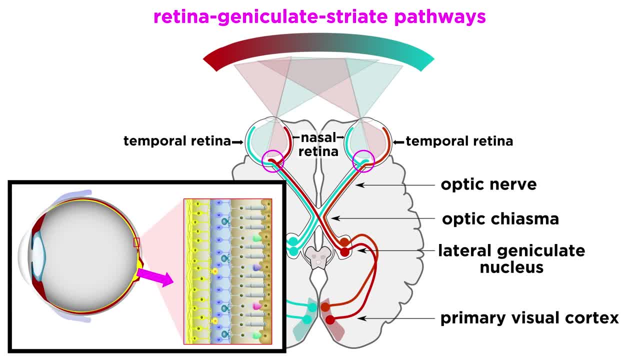 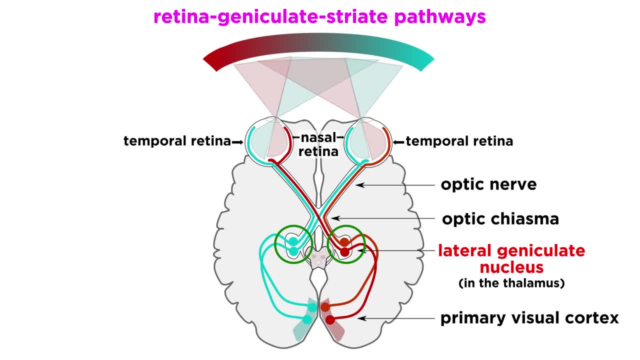 These begin with axons from the ganglion cells which leave the back of the eyeball and form the optic nerve. This will pass through the lateral geniculate nuclei found in the thalamus and then pass through the retina and then continue all the way to a region of the brain called the. 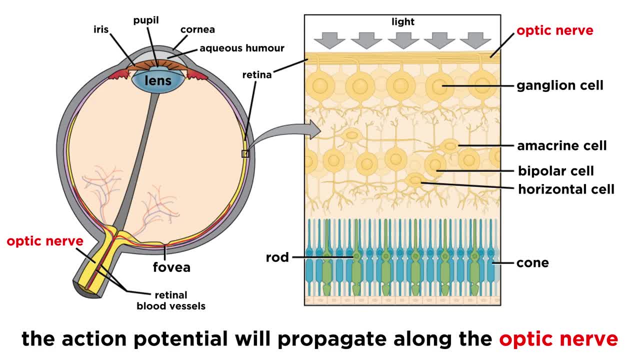 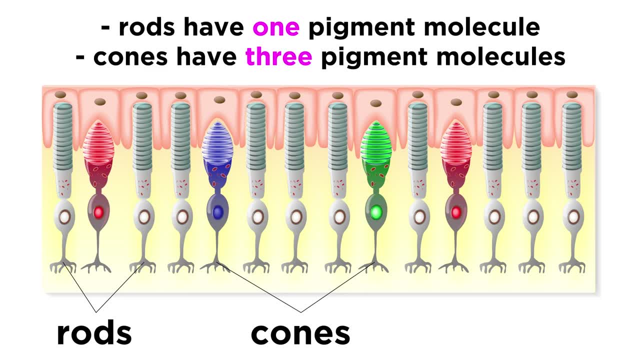 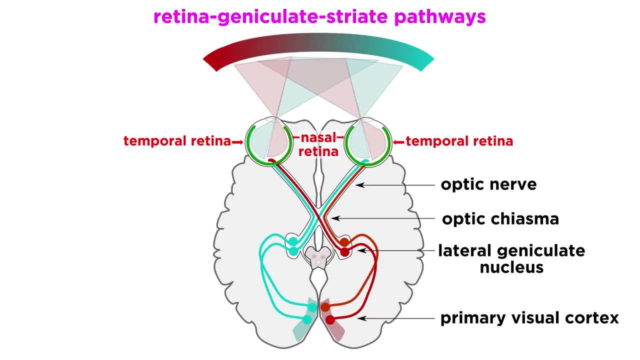 along the optic nerve. We should note that rods contain just this one pigment, rhodopsin, While cones contain three, which can act together in varying ways to allow for the perception of any color in the visible spectrum. Zooming out a bit, action potentials that start at the retinal ganglion cells will travel. 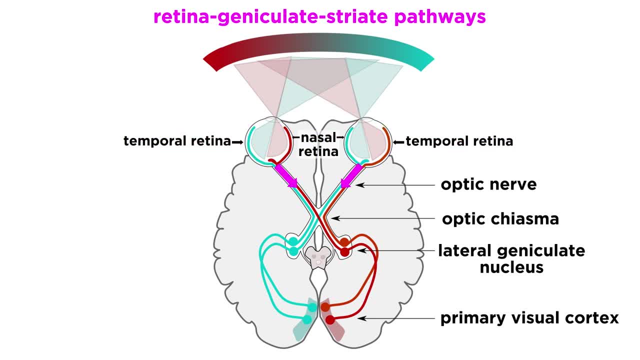 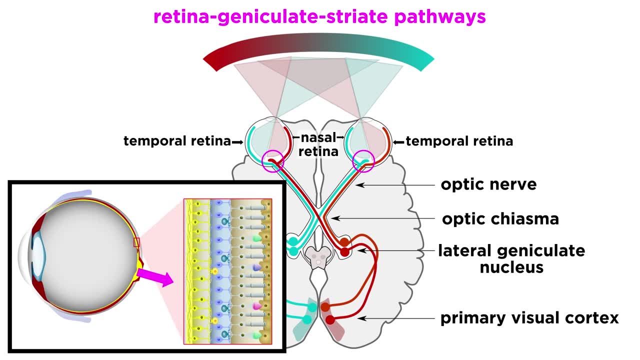 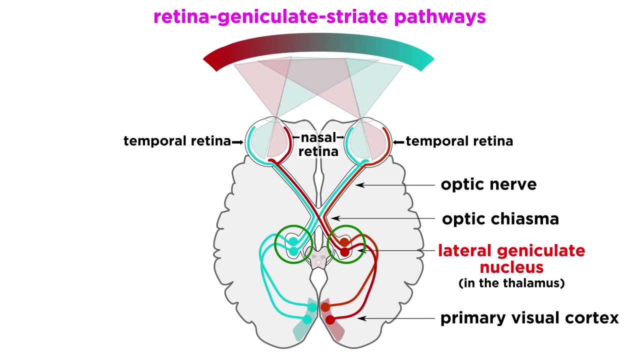 from the retina along retina-geniculate-striate pathways. These begin with axons from the ganglion cells which leave the back of the eyeball and form the optic nerve. This will pass through the lateral geniculate nuclei found in the thalamus and then continue. 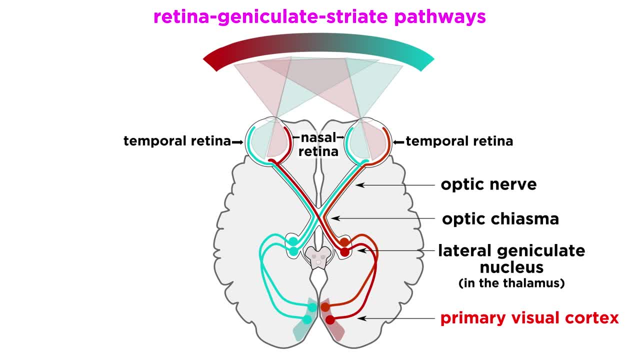 all the way to a region of the brain called the primary visual cortex, which is divided into left and right sections found in the left and right hemispheres of the brain. Notice that all the inputs from the left visual field are carried to the right primary visual. 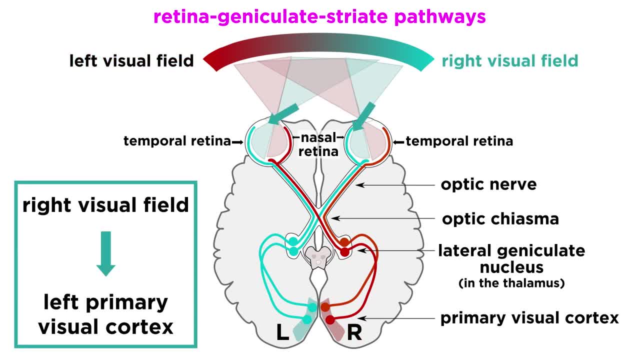 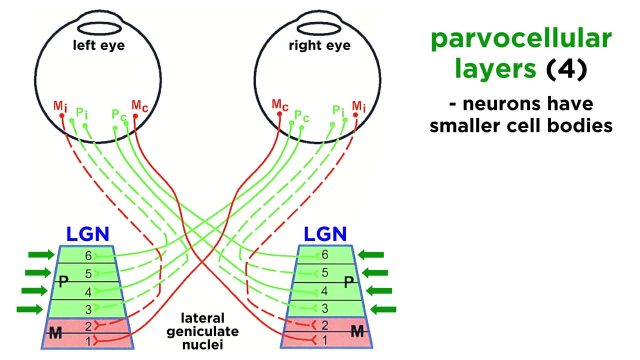 cortex. The left visual field is the primary visual cortex and the left visual field is the primary visual cortex. The right visual field are carried to the left primary visual cortex. Within these pathways we can also identify a few layers of neurons. There are parvocellular layers, also called p-layers, which are comprised of neurons with 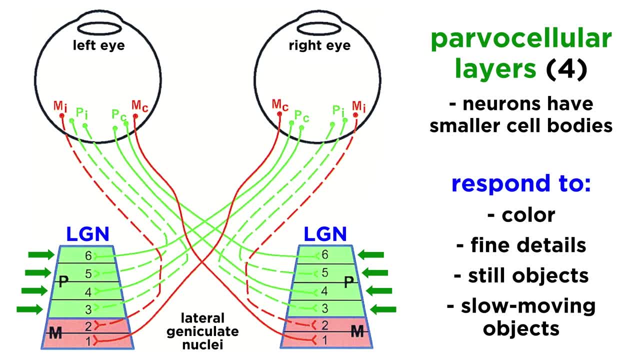 smaller cell bodies. These respond to color, fine details and objects that are still or moving slowly. Then there are magnocellular layers, or m-layers, comprised of neurons with larger cell bodies, which are more responsive to objects in motion. 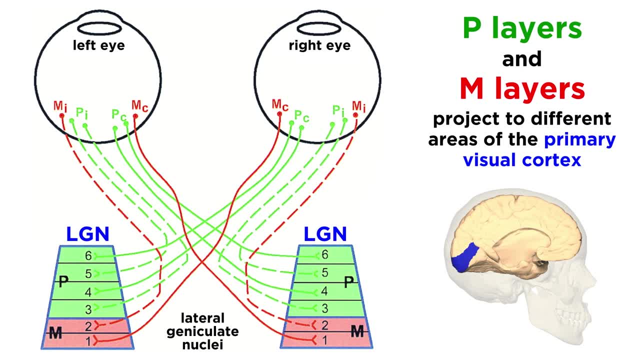 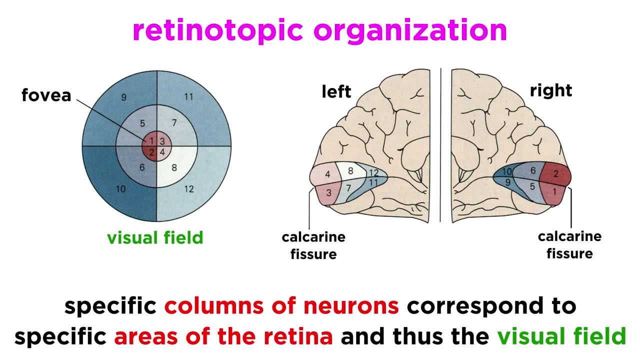 These layers project to different areas of the visual cortex. Another aspect of organization to the visual cortex is the way we can identify vertical columns perpendicular to the cortical layers themselves, which each correspond to a specific area of the retina called the retina. The retina is the area of the retina that is the most visible from a particular eye. 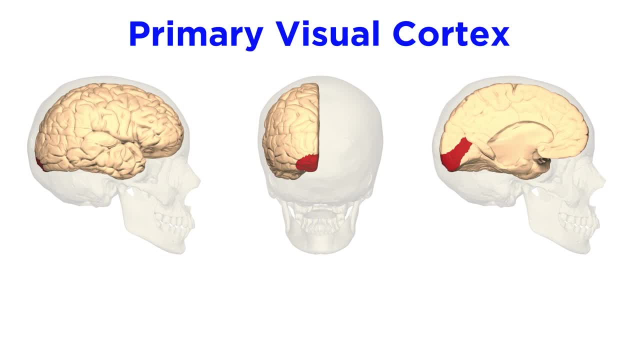 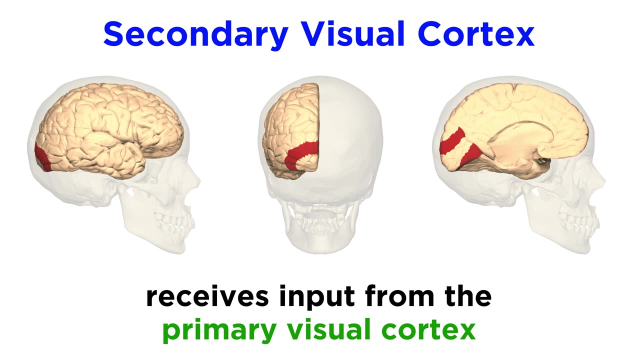 What other areas of the brain are involved here? Aside from the primary visual cortex, which receives most of its input from the lateral geniculate nuclei, we also have the secondary visual cortex. This is named as such because it receives input from the primary visual cortex. 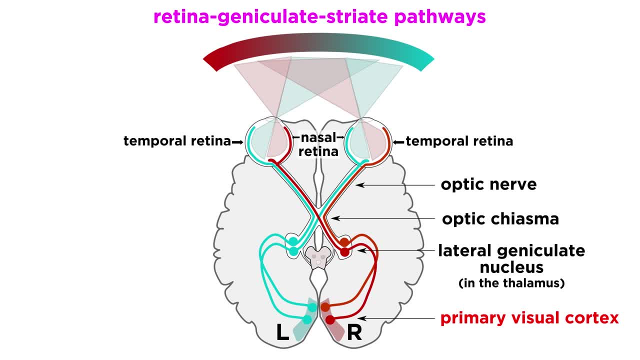 primary visual cortex, which is divided into left and right sections found in the left and right hemispheres of the brain. Notice that all the inputs from the left visual field are carried to the right primary visual cortex and inputs from the right visual field are carried to the left primary visual cortex. 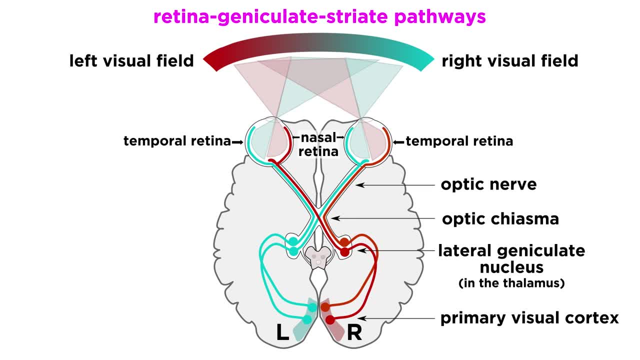 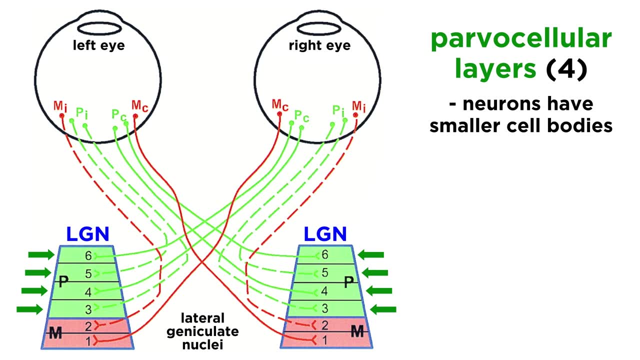 Within these pathways, we can see that the right visual cortex is the primary visual cortex and the left visual cortex is the primary visual cortex. We can also identify a few layers of neurons. There are parvocellular layers, also called p-layers, which are comprised of neurons with 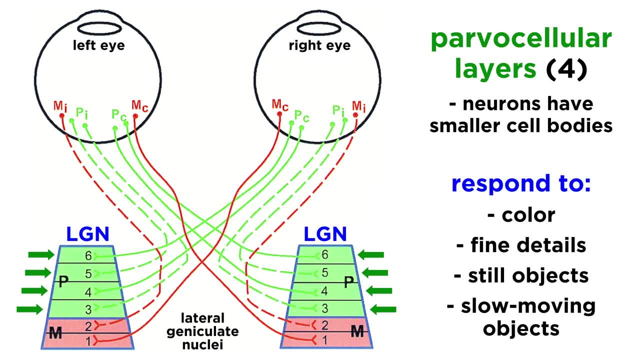 smaller cell bodies. These respond to color, fine details and objects that are still or moving slowly. Then there are magnocellular layers, or m-layers, comprised of neurons with larger cell bodies, which are more responsive to objects in the brain. 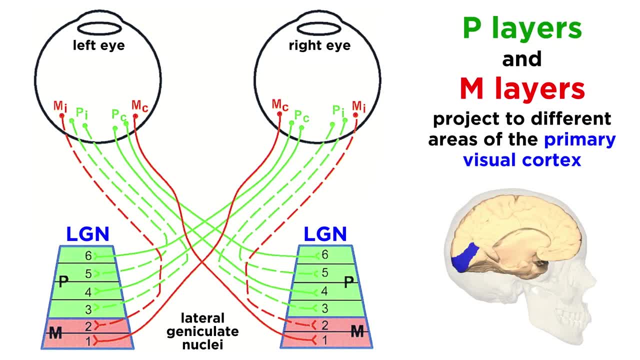 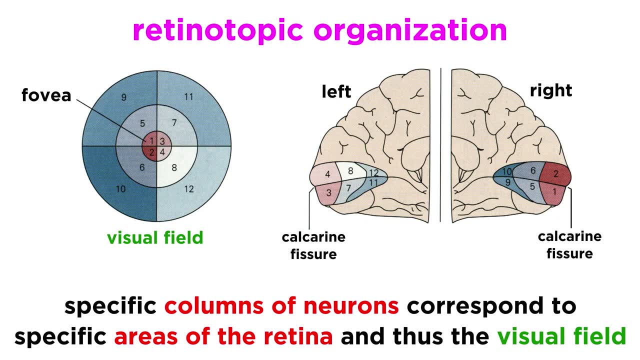 These are also called visual cortex layers, and these are the layers that project to different areas of the visual cortex. Another aspect of organization to the visual cortex is the way we can identify vertical columns perpendicular to the cortical layers themselves, which each correspond to a specific 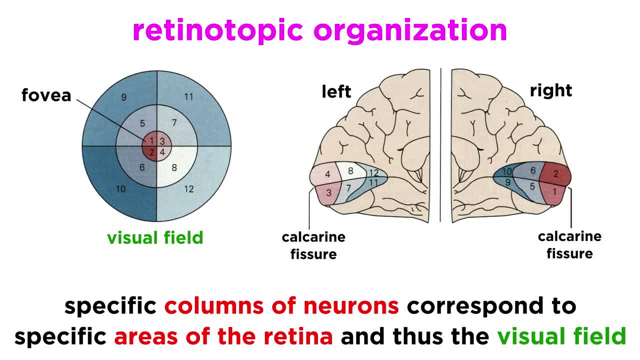 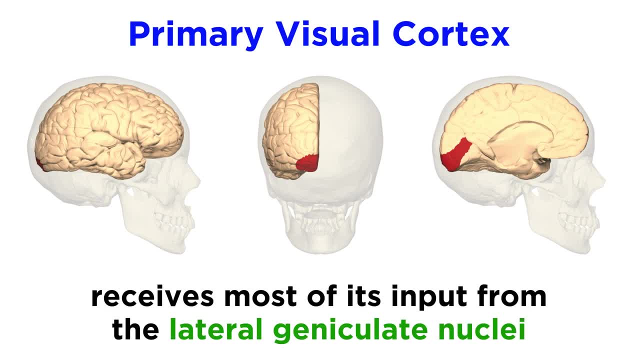 area of the retina from a particular eye. What other areas of the brain are involved here? Aside from the primary visual cortex, which are the main visual cortex, we also have the retinal cortex, which receives most of its input from the lateral geniculate nuclei. we also have the 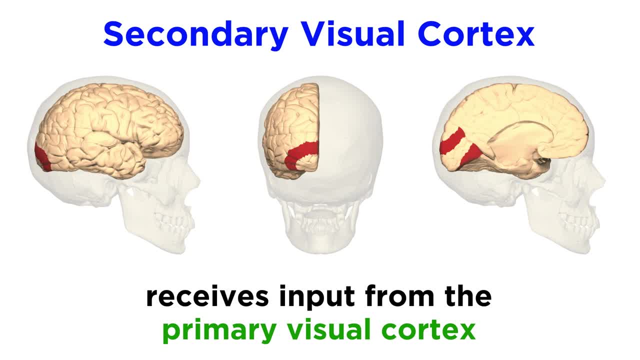 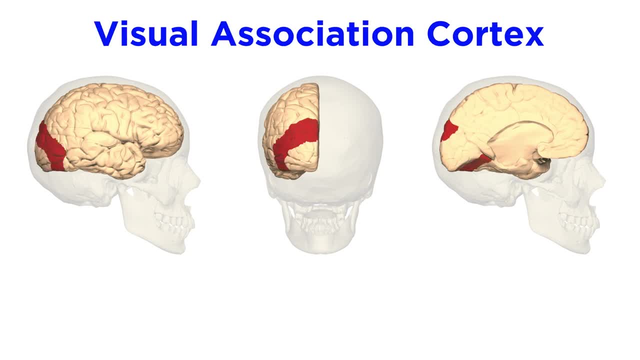 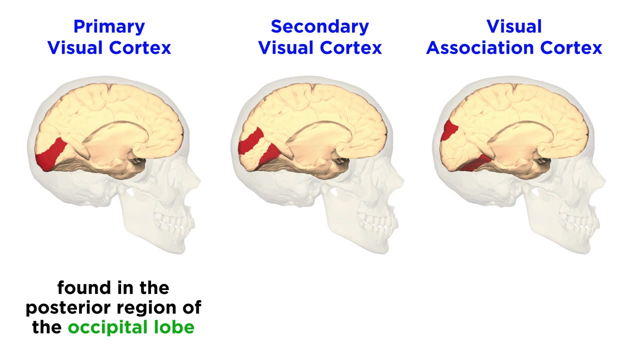 secondary visual cortex. This is named as such because it receives input from the primary visual cortex. Then there is the visual association cortex, which receives input from the secondary visual cortex as well as other areas of the brain. To help distinguish the locations of these regions within the brain, we can see that 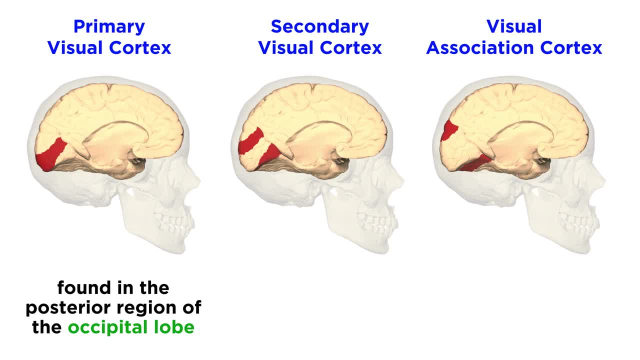 the primary visual cortex sits in the posterior region of the occipital lobes. The secondary visual cortex can be found in the pre-striate cortex which surrounds the primary visual cortex, as well as the inferotemporal cortex, which is found in the inferior temporal. 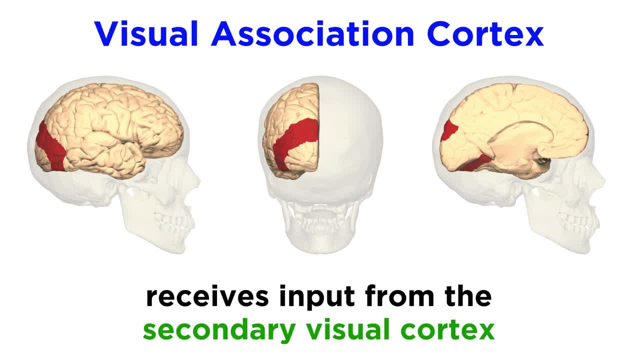 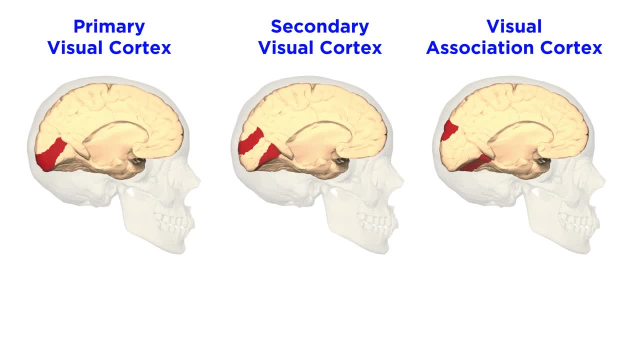 Then there is the visual association cortex, which receives input from the secondary visual cortex. This is known as the visual association cortex. To help distinguish the locations of these regions within the brain, we can see that the primary visual cortex sits in the posterior region of the occipital lobes. 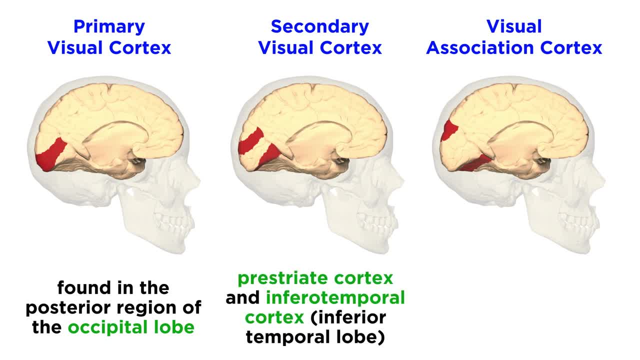 The secondary visual cortex can be found in the pre-striate cortex which surrounds the primary visual cortex, as well as the inferotemporal cortex, which is found in the inferior temporal lobe. The visual association cortex is found largely in the posterior parietal cortex and also 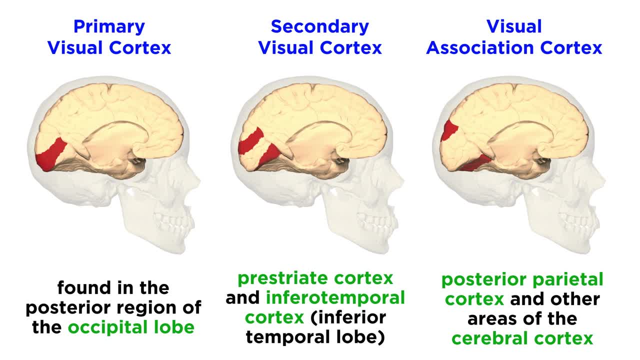 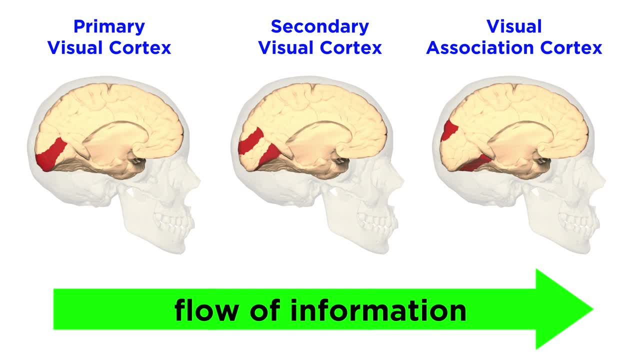 distributed around other areas of the cerebral cortex. As we said, the hierarchy is such that visual information goes from the primary cortex to the secondary, then to the association cortex. These other two areas of the brain are responsible for visual analysis, or the interpretation. 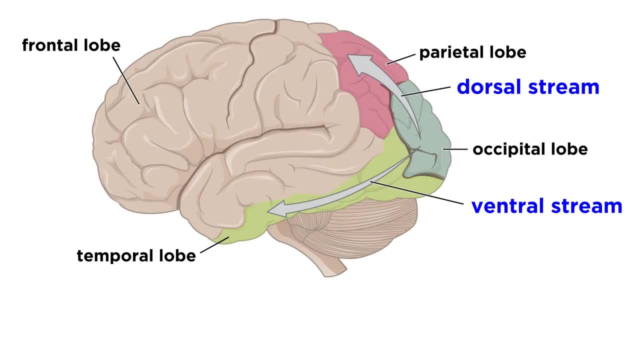 of the information brought to the primary cortex, The visual association cortex is also found in the posterior parietal cortex and also distributed around other areas of the cerebral cortex. This information travels to these regions via the dorsal stream and the ventral stream. 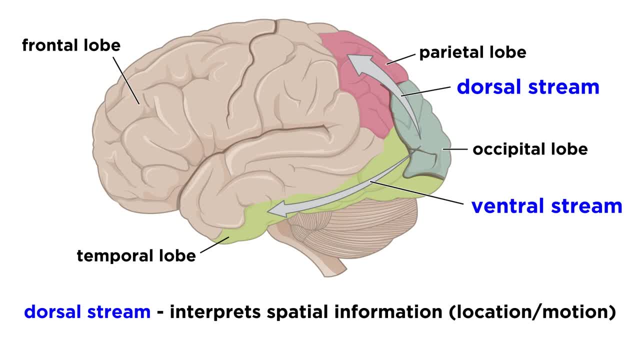 Roughly speaking, neurons in the dorsal stream interpret spatial information like the location of an object and its motion, while the ventral stream is for object characteristics like color and shape. The dorsal stream flows from the primary visual cortex to the dorsal pre-striate cortex. 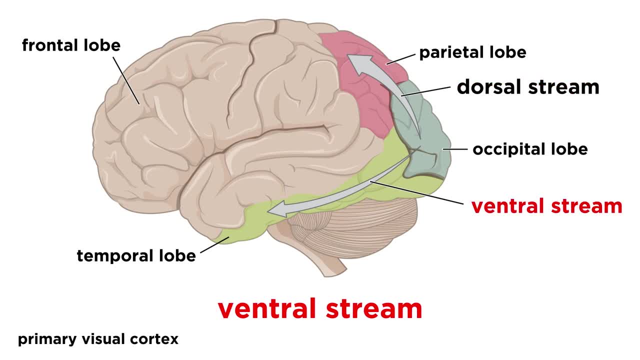 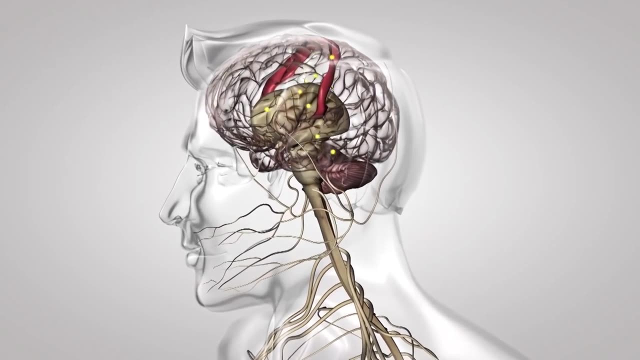 to the posterior parietal cortex, While the ventral stream flows from the primary visual cortex to the ventral pre-striate cortex, to the inferotemporal cortex, as is shown here. There is much more to discuss regarding how the brain processes visual information and. 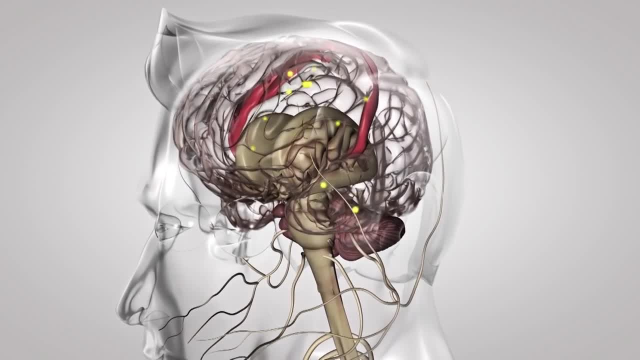 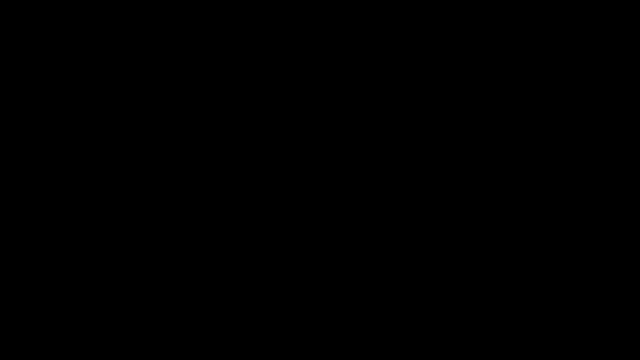 we will elaborate on all of this in the future, but for now we will have to stop here and move on to some other topics, so let's check out the other senses next. Thanks for watching, guys. Subscribe to my channel for more tutorials. support me on patreon so I can keep making. 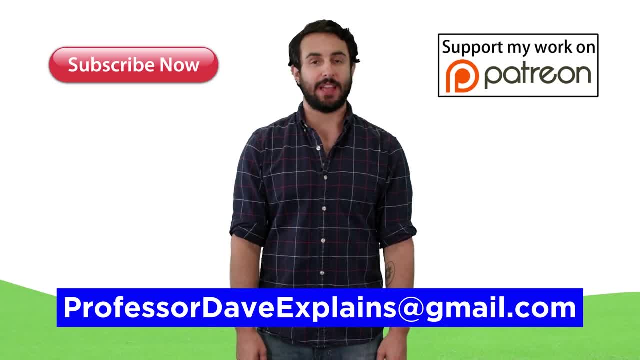 content and, as always, feel free to email me professordaveexplains at gmail dot com.